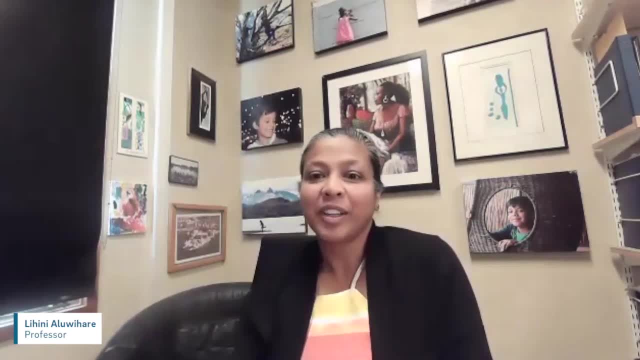 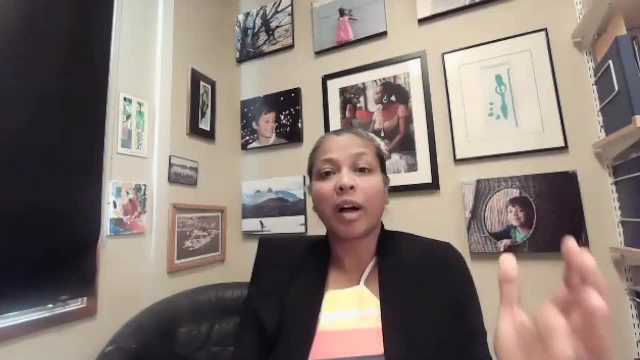 of the distribution of carbon and nitrogen in the ocean And it's also the study of the distribution of chemical elements in seawater. And we are trying to understand what are the sources of these chemicals, what are the sinks, the removal processes and also what 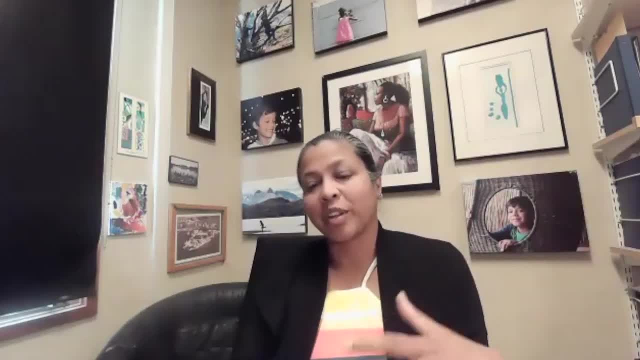 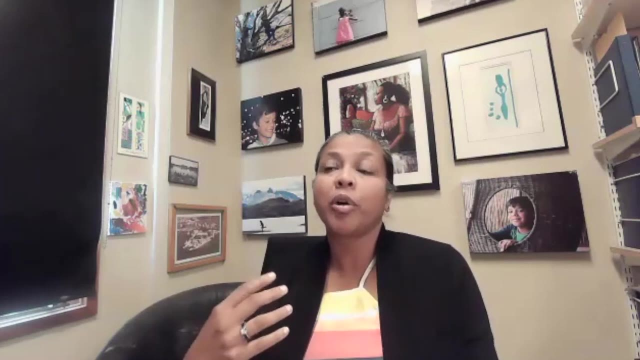 transforms them and how those transformations impact their lifetime in the ocean. And understanding kind of all these aspects of elemental cycling in the ocean allows us to understand or predict how these chemicals and their distributions in the ocean will respond to pulses and processes and how they're going to affect the life cycle of the ocean. And so that's kind of the 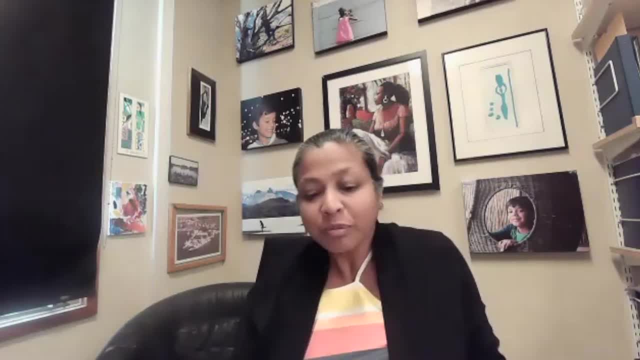 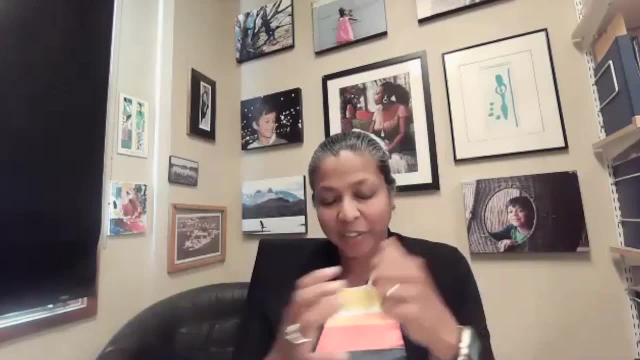 first part And then the second part is: you know what are the processes of change? things like global climate change, And so, in this vast space, I've developed a particular interest in the part of chemical oceanography that's influenced by living organisms, and specifically how. 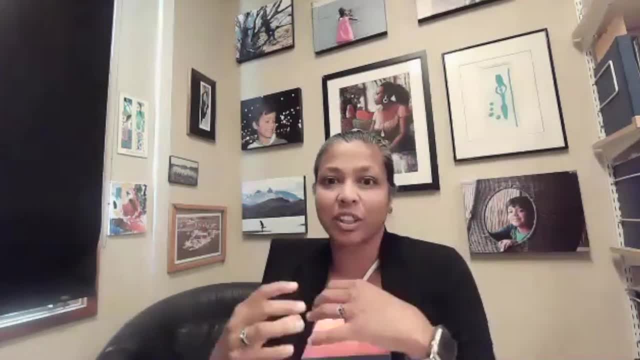 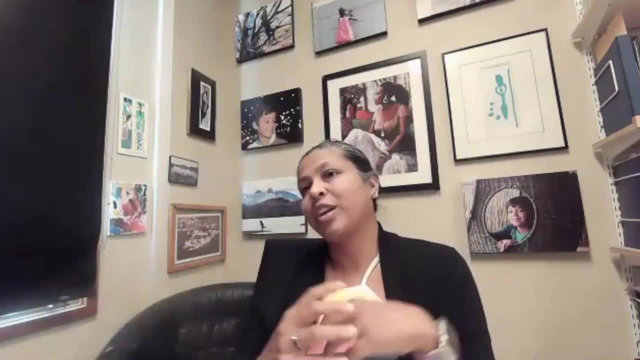 living microorganisms interact, as you said in your introduction, with the carbon and nitrogen cycles and then how carbon and nitrogen moves back and forth between all the compartments. you know the water column, the particles, the organisms and the sediments, And so 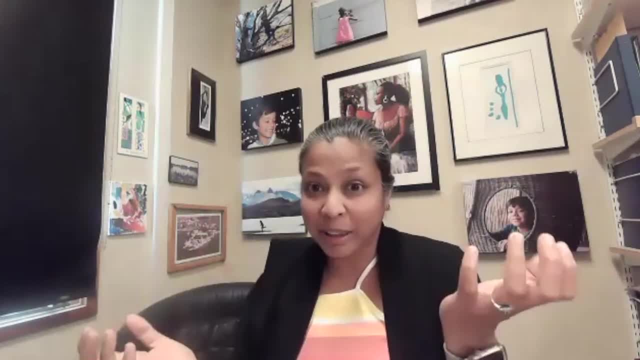 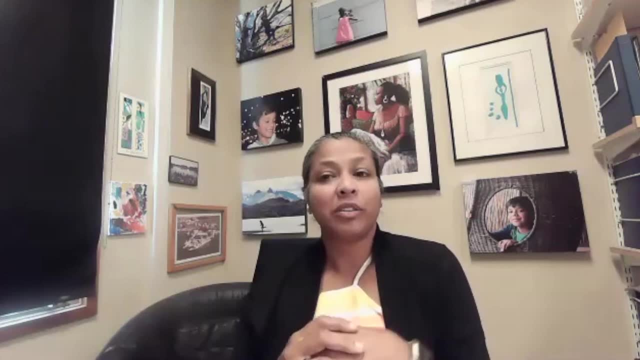 I'm very fortunate because to do my research I have to be in the water somewhere. And in coastal environments, you know, we see both the complexity of how organisms modify their environment, but we also see the anthropogenic fingerprint, as you described, And then in open ocean environments. 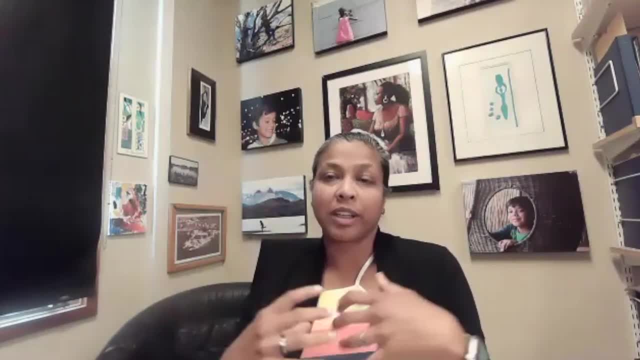 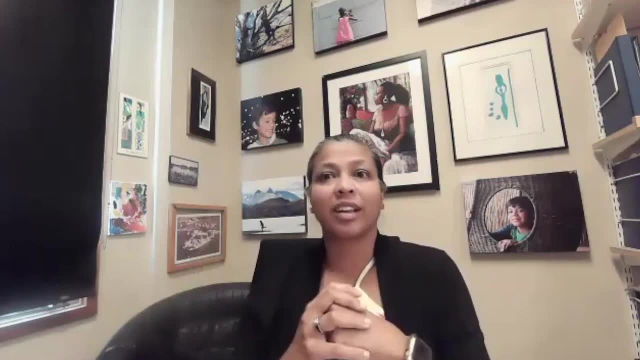 we can really observe how microorganisms structure their interactions in the absence of environmental changes, And so I think that's really important. And then you know, I think that's very important. But when I first started working in this field, I learned about the 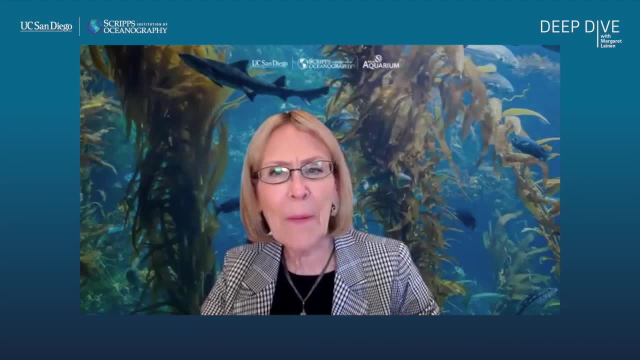 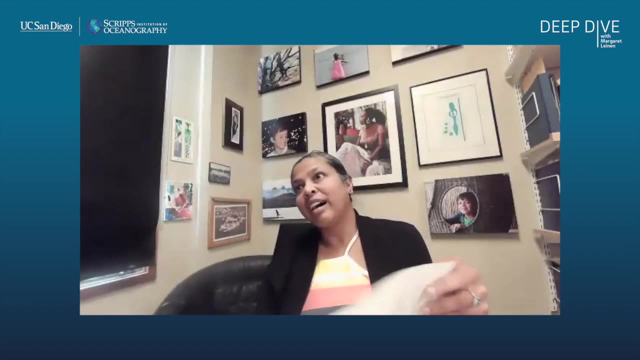 likelihood that- and this is actually what I learned from a project. I did not go to the 一起, but I did not know about anthropogenic propellants and anthropogenic contaminants but how they structure the interactions through the chemicals that they make. So what kind of tools do you use to study carbon cycling? 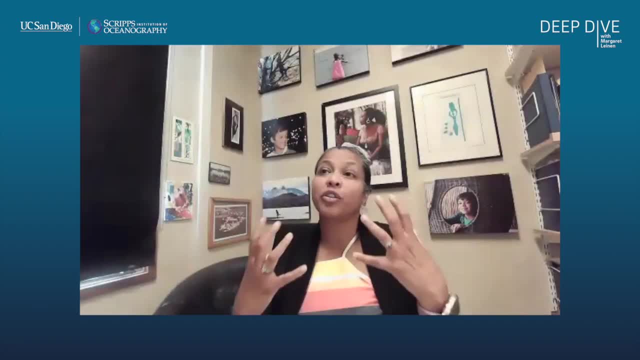 Yeah, so we are. you know, I'm interested in carbon and nitrogen, carbon and nitrogen, And I want you know. so what's the complexity of the of the chemicals that participate in these cycles and when we're thinking about the interaction of these cycles with organisms? you've got the vast and just the. 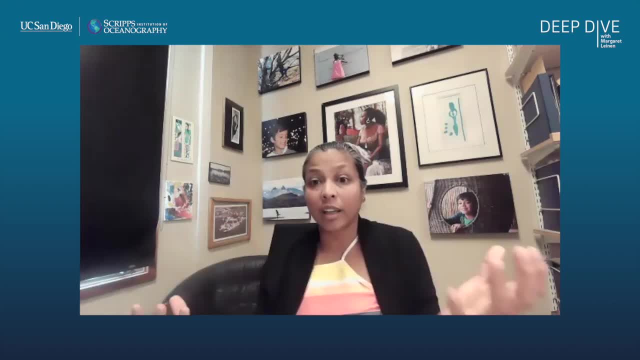 vast complexity of what's genetically encoded. so we're talking about millions of different compounds. but once these organic molecules get into the ocean, they are transformed by light, they're transformed by their interaction with particles, with the interaction with different kinds of reactive chemical species, and so we know that this complexity is important. it it enables 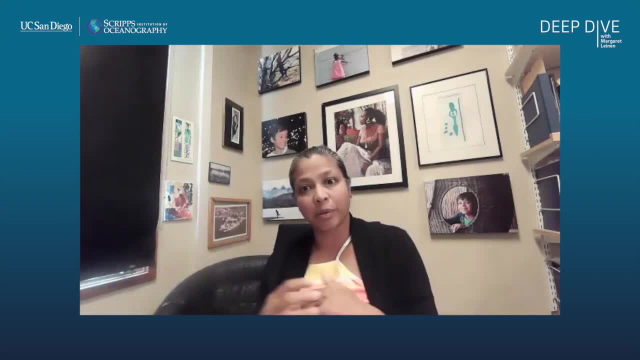 organisms to perform their day-to-day activities. it enables them to interact with one another and we know that these transformation processes are important in terms of determining how long these compounds might live in the environment, so sort of the storage capacity within this reservoir for nitrogen. so that's really the major challenge, right? how do we address this? complexity and a lot. 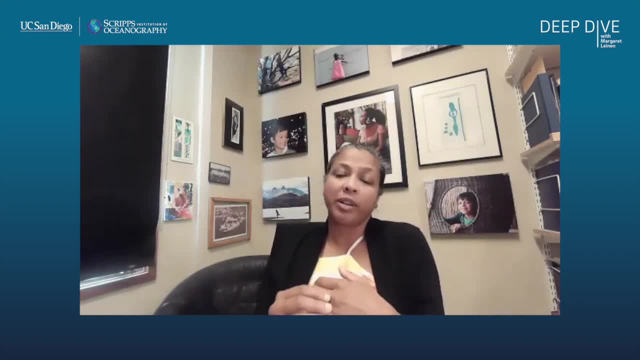 of my work has to do with developing advanced analytical methods. to really kind of pick apart: what are the molecules that are in there? what are their structural moieties? what makes them special? how might that allow us to understand what these molecules do in the environment, but also 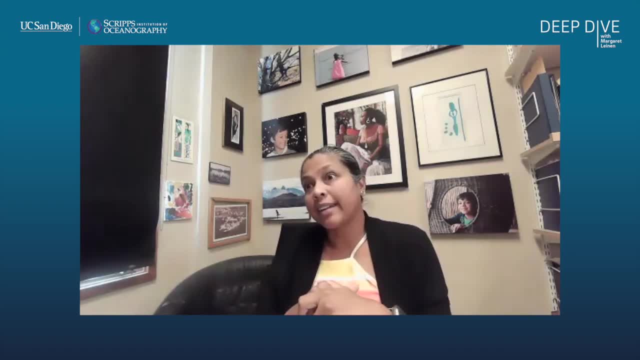 within organisms. another aspect of that is the ability to use tools like stable and radioactive isotopes, because those give you a whole different view into how, what environments these compounds are produced in, how those compounds were transformed, and it's one of the things that i find really fascinating that you can use isotopes of individual molecules in. 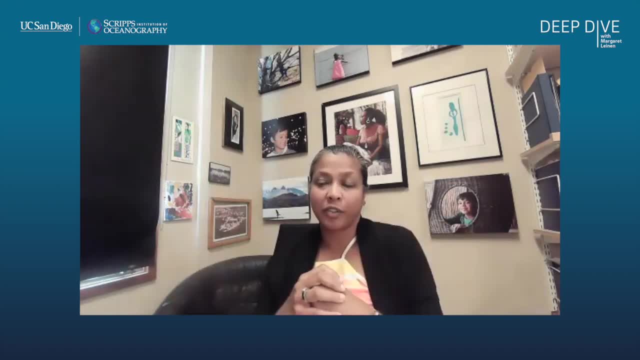 seawater to understand kind of the whole history of something. and within that space there's also the use of radioactive isotopes. so using radioactive isotopes to get at the time scale- and that's really important when we're thinking about how the ocean responds to change- we need to understand rates at which these compartments 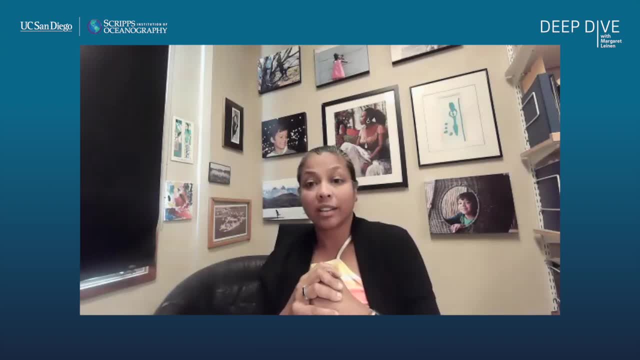 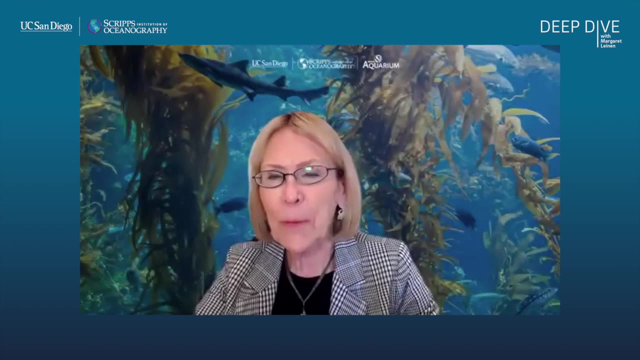 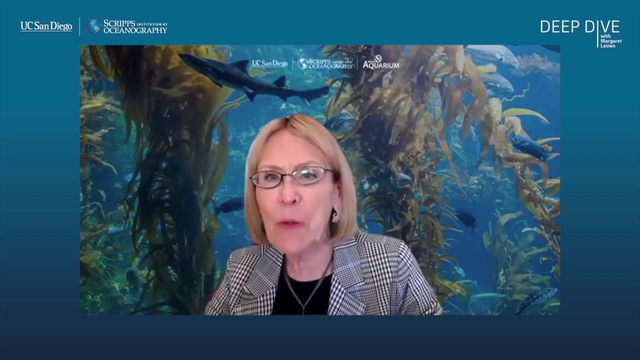 interact with each other, and so radioactive isotopes really give us this additional power that we can't get with stable isotopes. so both of those together are things that i really enjoy applying. so you you mentioned that, geçイ to asked earlier about how you used the tools in this conceptual sense. 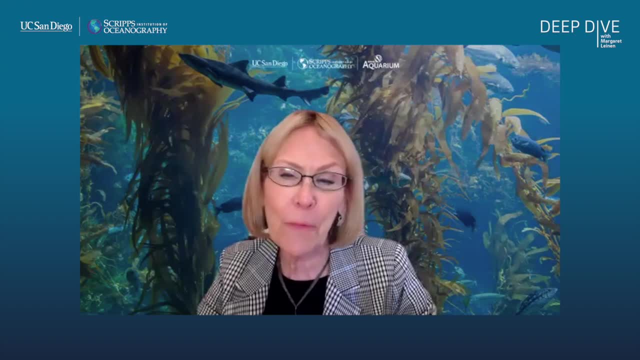 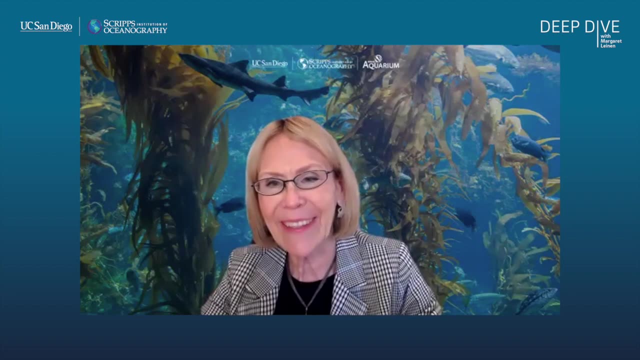 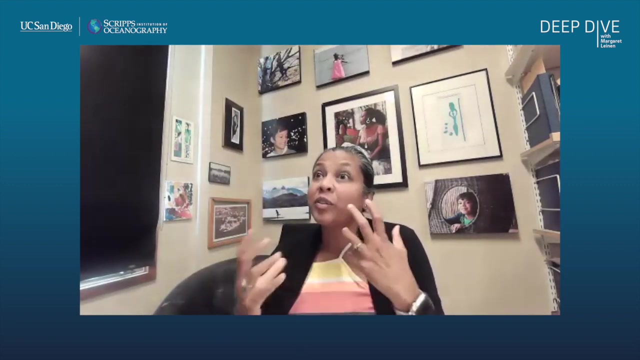 so most people think of tools as instruments and sensors and so forth. what kinds of infrastructure and instruments do you use to do the work right? so you know the i spoke of the complexity, which, of course, um, um is is the thing that i think about all the time, and some people i um 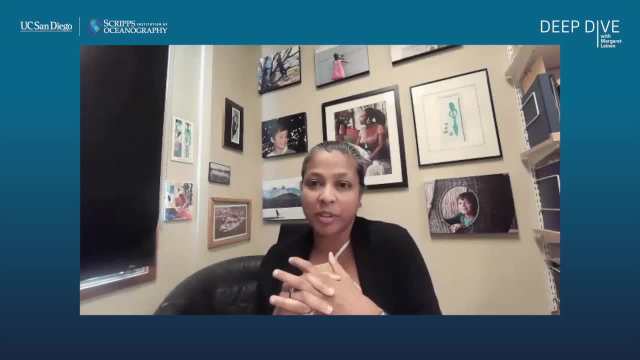 that my lab looks a little bit like a crime scene investigation TV show, because we have some of the same instruments, because it's, you know, you're still dealing with the complexity. you're trying to, you know, pick a particular signal out of all the different environmental signals. the sample: 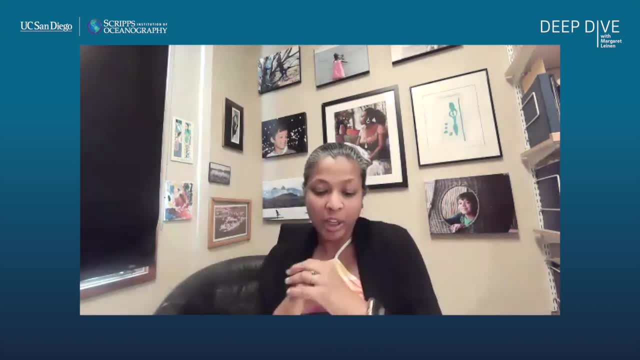 might have in a particular crime, And so we're thinking exactly about that, And one of the things that we might want to do, for example, is, you know, is tell the difference between something that might have come from a naturally produced, that might be naturally produced, and 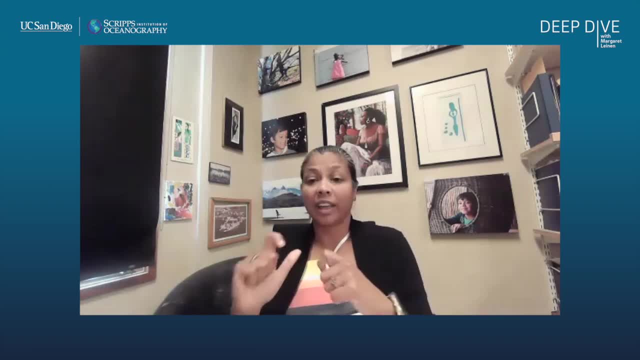 something that might be anthropogenic. So sometimes you can use the chemical handles to tell that. So, for example, if we're thinking about something like DDT, we know that they have chlorine. it's a molecule that has chlorine in it, And so we might just 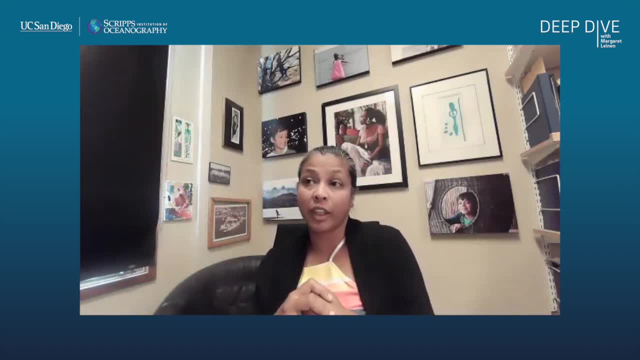 look specifically at the chemical handles and we might look specifically at the chemical handles for that handle. we might detect specifically for that. But then you might have compounds that can come from multiple sources, And that's when we can deploy tools like isotopes, because 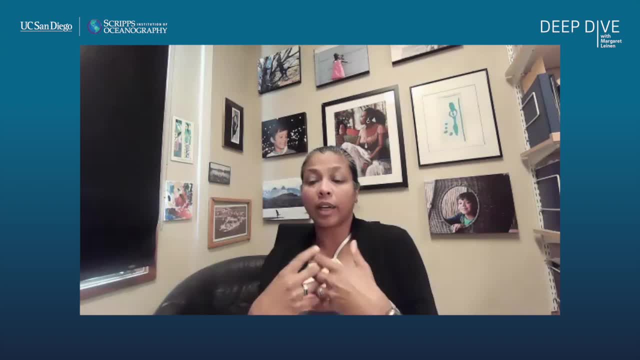 you know, I spoke about radiocarbon, And if you have an anthropogenic compound in the environment, it's what we call radiocarbon dead. it's devoid of radiocarbon because it was synthesized essentially from petroleum, which is, you know, millions of years old, and the C14 has decayed. 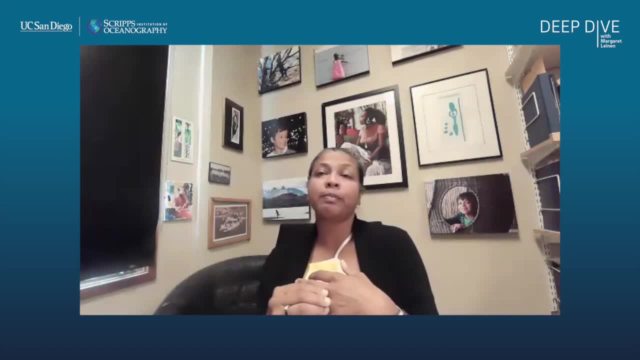 away, Whereas something that's produced by an organism today in the environment has a has a different chemical, different isotope composition. One other way that we use radiocarbon was there's a, there's a gradient in the C14 content or the radiocarbon content of. 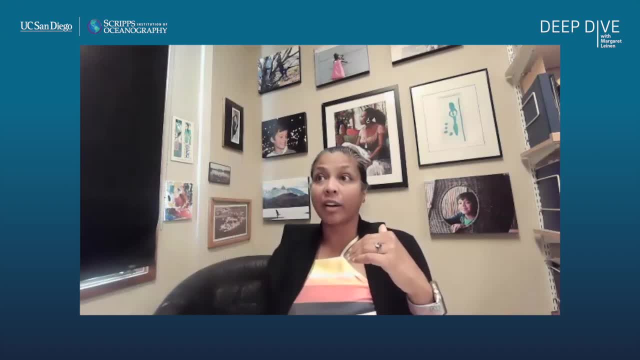 inorganic carbon with depth in the ocean, And so we use that gradient to actually understand how microorganisms in the deep ocean are making a living. So you isolate a particular molecule- because that's what we like to do- like DNA or a particular living organism, and we isolate a. 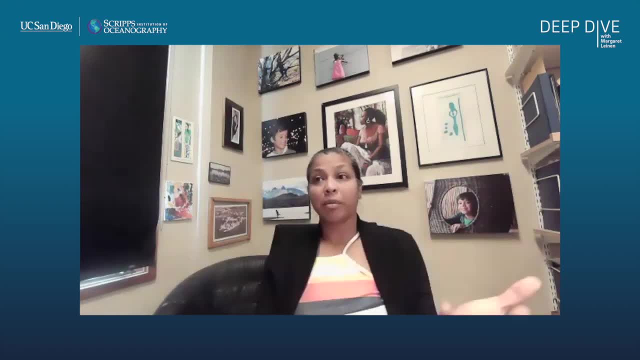 particular molecule- because that's what we like to do- like DNA or a particular living organism, And then we can measure its isotope content and say: oh, this organism is getting its, even though it's living in the deep ocean. it's getting its food from the surface or it's actually making its food in the environment. 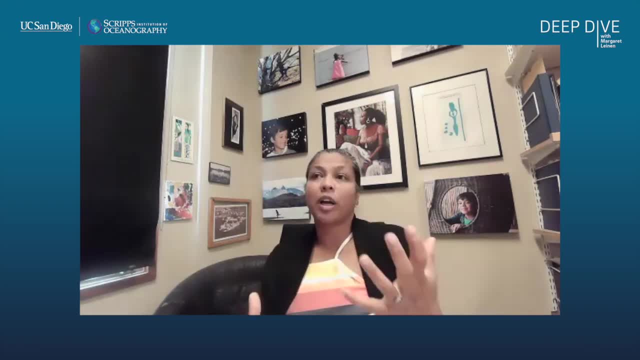 So both capitalizing on these advanced mass spectrometry tools that allow us to kind of unravel the complexity of these molecules, and then combining that with things like isotopes allows us to really get a very rich picture of not just what's there but how those things are moving through the ocean system. 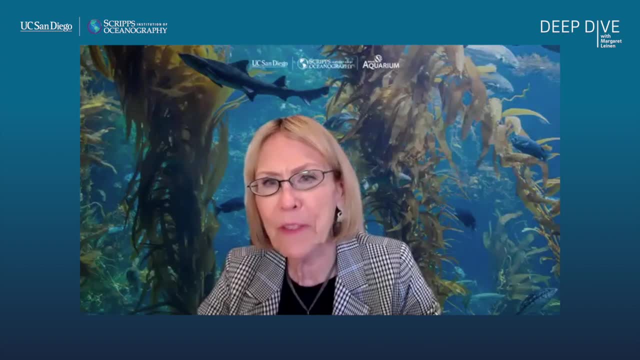 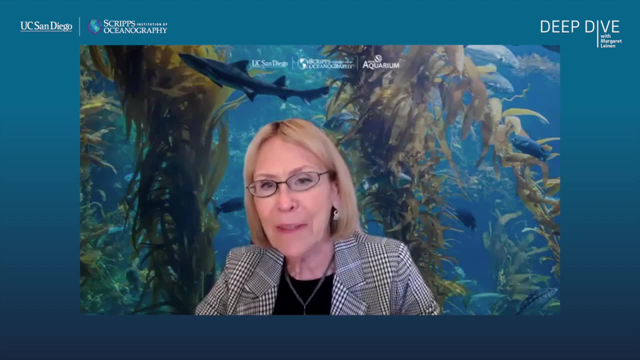 Can you give us an example of something that moves quickly versus and moves rapidly through the system versus something that sort of hangs around for a long time? Yeah, that's a great question. It's actually what I spend my time thinking about. 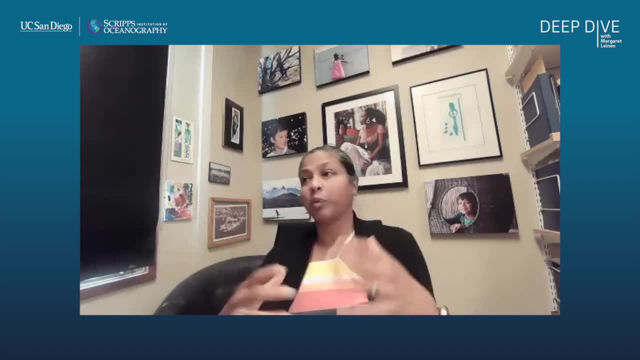 So you can think of organic. you know, we often think of when we think about fertilizer or something we think about nitrate and phosphate, these inorganic components, But there's a lot of organic nutrients that are essential. So certain microorganisms- in fact the most abundant microorganisms- have a very streamlined genome. 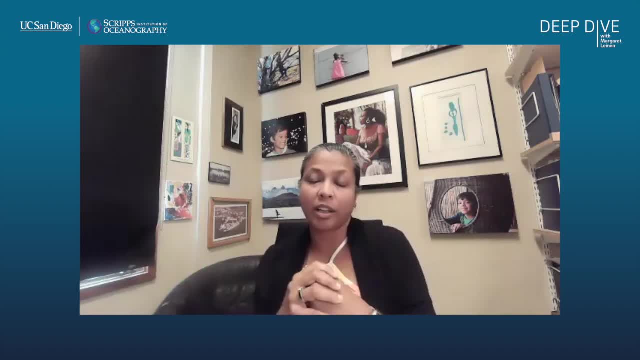 So they don't actually have the capacity to make a lot of the metabolites that they need, So they might take organic sulfur compounds. Vitamin B12 is a great example. We Don't think about that a lot But, yeah, most a lot of phytoplankton don't make vitamin B12.. 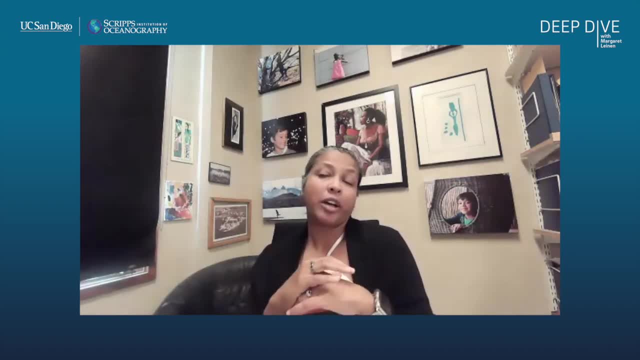 So they rely on their microbial partners And there's a lot of examples of molecules like that And we're still learning, really because we haven't been able to unravel the complexity. So vitamin B12 will be something that's very rapidly taken up from the environment. 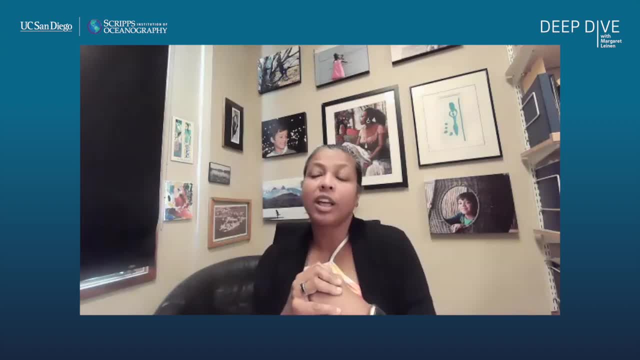 You're not going to find high concentrations of that sitting around in the water, whereas some of these anthropogenic components- those are not There- are Persistent by nature, And so we might expect them to accumulate on long timescales. And, naturally speaking, you know when we think about oil, and you know especially oil and even coal. these are organic molecules that were transformed in particular ways such that they're really- maybe they're- not energetically favorable. you know an organism. 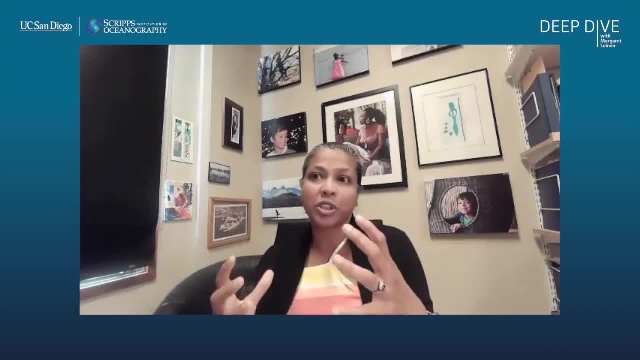 Why would you know? in a, in a fairly desert, like ocean, Why would they expect to expend the energy to eat something that's not going to give them much In return? and so we see compounds like this, and that's actually a huge part of what I'm trying to. really, this is sort of my discovery part that I've been working on for my whole career- is really trying to really trying to describe what it is. that. what kind of chemical signature would tell us whether an organic compound is good to eat? 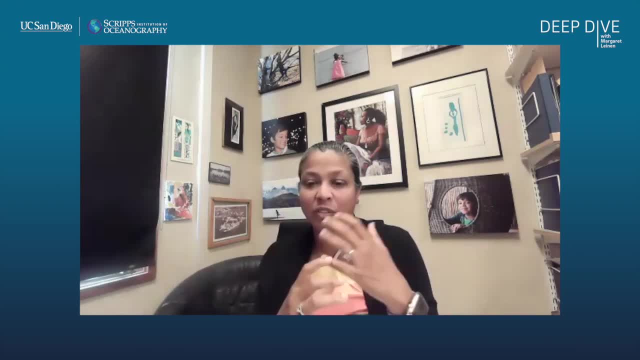 You know they often people use like the analogy of steak and a tire or something like that. You know what are the chemical signatures that make something a tire. you know that nobody wants to eat. So those are some examples. Or ice cream and a tire. 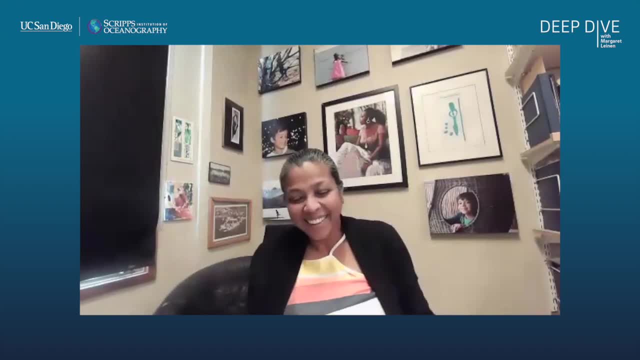 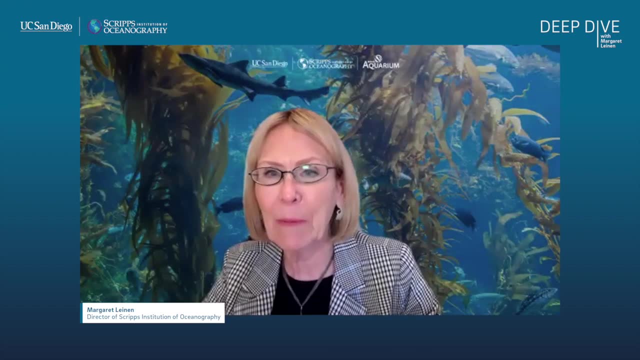 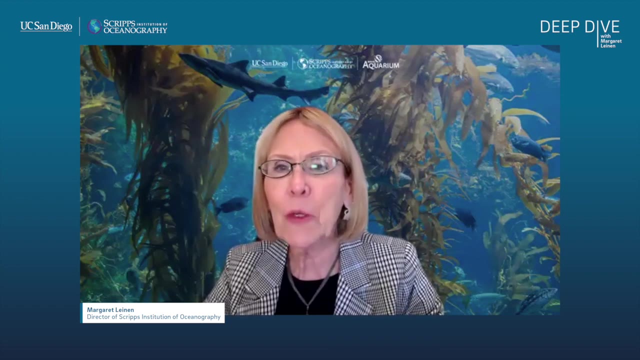 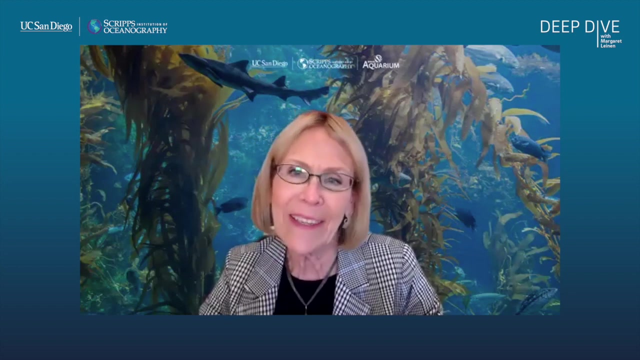 Yeah, that's a better one. So you were. you said that many people said your lab looks like a crime scene investigation. So that brings us back to this idea of human fingerprints. So in your crime scene investigation, what have you found as you looked for those fingerprints? 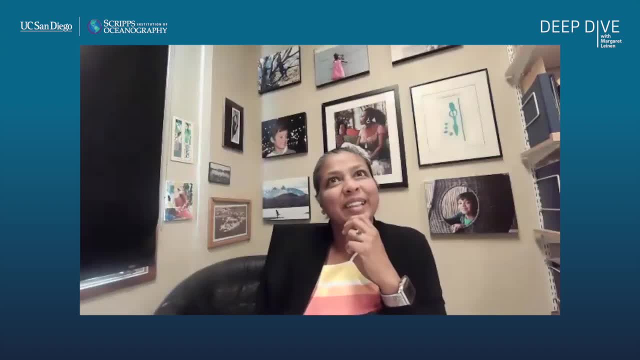 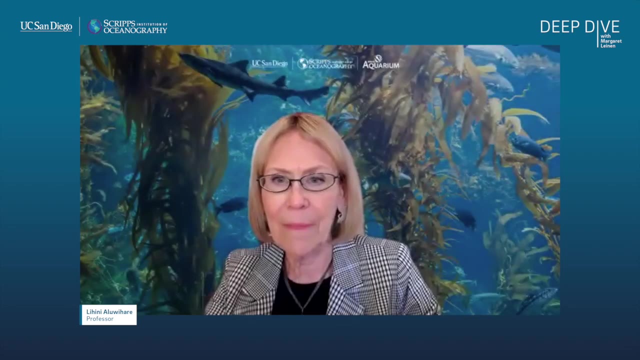 Yeah, it's a. it's a. it's been really interesting because, you know, when you go into this coastal environment, you have all these different signatures that you see. you know, we collect the samples, we analyze them with our tools and there's all this information. 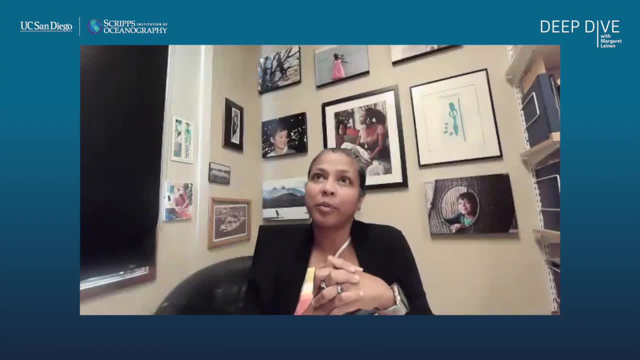 And so how do we start to unravel? And so how do we start to unravel some of these questions? So actually, I've been thinking about this very recently because I was born in Sri Lanka And yesterday or two days ago, a container ship caught fire outside the port of Colombo, which is the major city there. 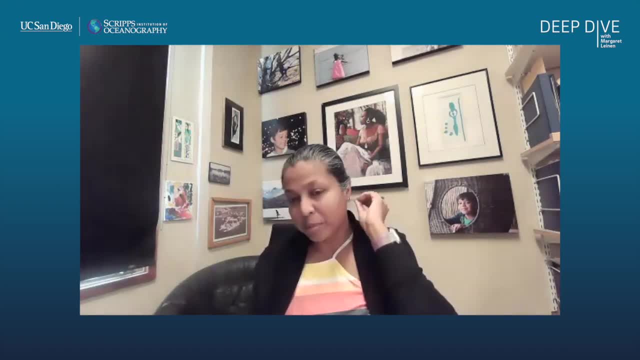 And I know a very famous marine biologist there, Asha DeVos, and she called me and she said: what you know, what, what, what do you think is the impact of this? And and so she started telling me what was in the 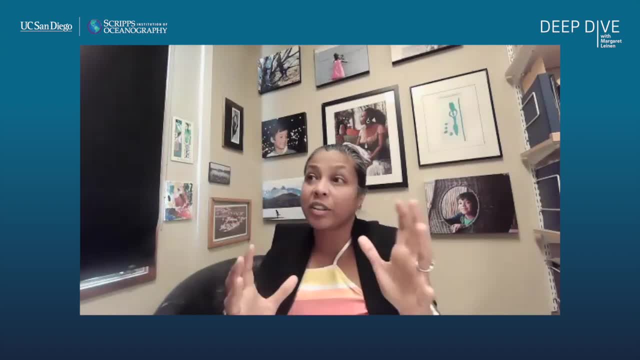 The container. So there were all these, you know, there was acids, but then there was cosmetics, And then, of course, there's the fuel oil, Right, And so you know, one of the things we have to think about, you know, is: what are you know what? what, what do we as humans put into this environment? 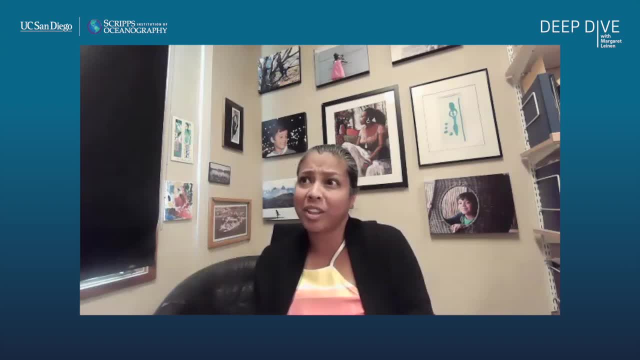 And what? what are the impacts on these ecosystems? How do those things even get into the environment in the first place? And so you know, a lot of the things that we found are what you would expect to find: things like persistent organic pollutants. 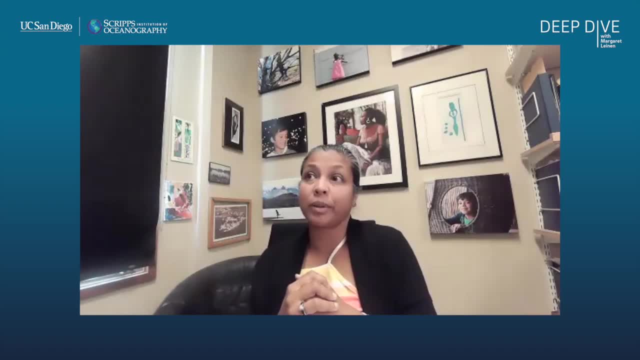 So the DDT suited compounds, as an example, PCBs, these brominated compounds, these flame retardants that were manufactured until very recently. But then you also start to find things like cosmetics or or drugs. or you know, during Christmas time you find cinnamon and vanilla right in the, in the wastewater. 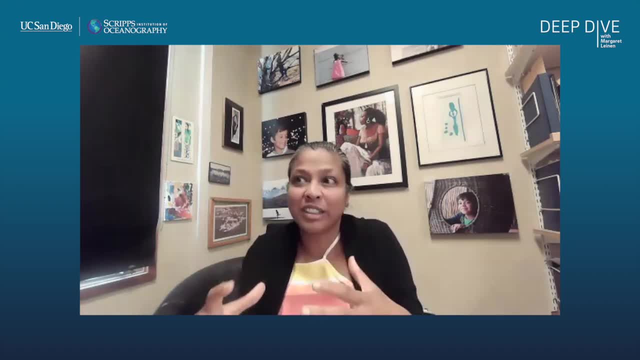 So you know, our, our connection to the environment is so profound, And you see that even externally, And so you know, one of the things that we have to think about, you know, is how do you ensure that these things are expressed in these, really these individual, at the individual molecule level? 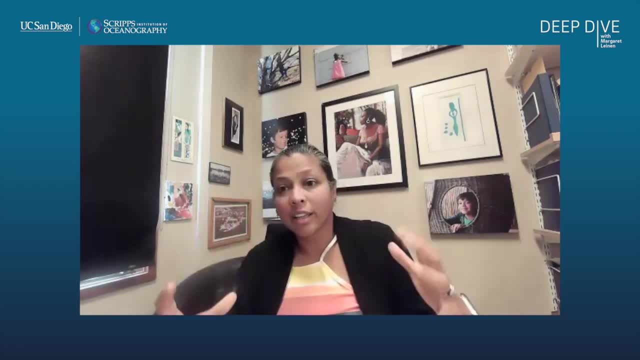 But one thing that we also discovered, or that others have also discussed this, is that a lot of the times when we're looking for anthropogenic signatures, where we're monitoring particular things- So, taking the DDT example, my collaborator Eunha Hoa, SDSU- she was leading this charge- 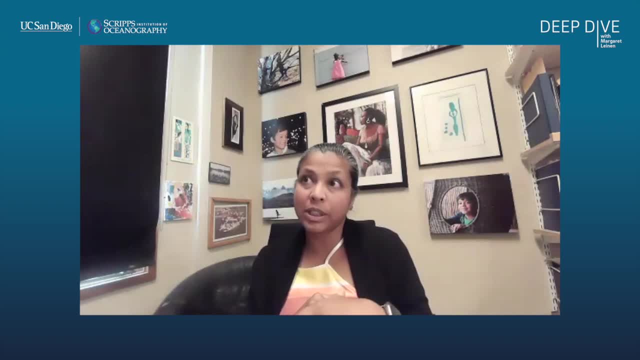 And what we found when we looked at Different samples- local region- was not only that, it contained, you know, over 300 compounds that were of anthropogenic origin, but it's only a fraction of those compounds are actually monitored or actually being detected. and the same with the DDT suite of compounds: there were more than 45 compounds that we could connect. 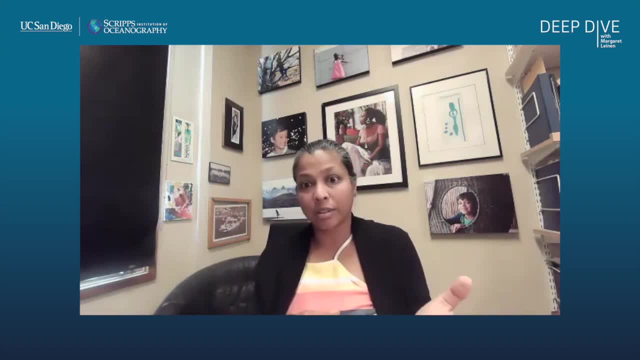 back to DDT either through the manufacturing process, and so if you were to, if you were to take sort of a- you know, if you put the blinders on and you're only looking for certain things, you know that's all you're going to find right. and so one of our really innovations has been 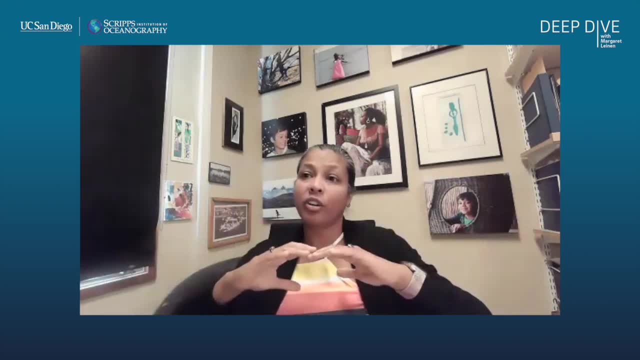 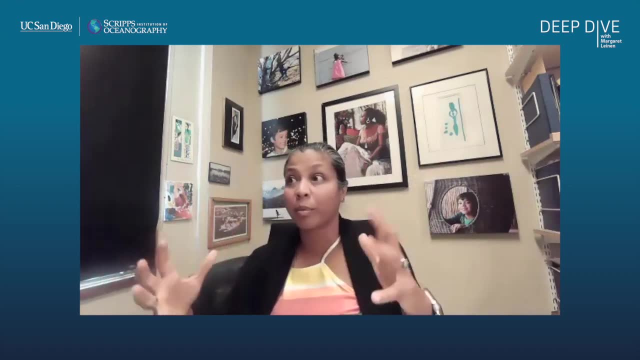 trying to do what we call this untargeted approach, really trying to get a snapshot of the whole, which is not easy and and you know we- we had a lot of pushback because it's hard to come up with even big data analysis methods to really sift through all this information, but it really gives. 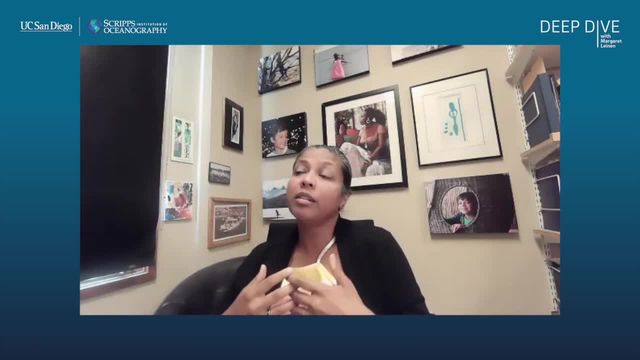 you a profoundly different insight. profound a different insight into what's going on. and just to go back to the DDT question, just because it's a interesting example, there are certain chemicals that are that we think are included in the technical mixture, that are in pretty small amounts, but when we go and look in the blubber, 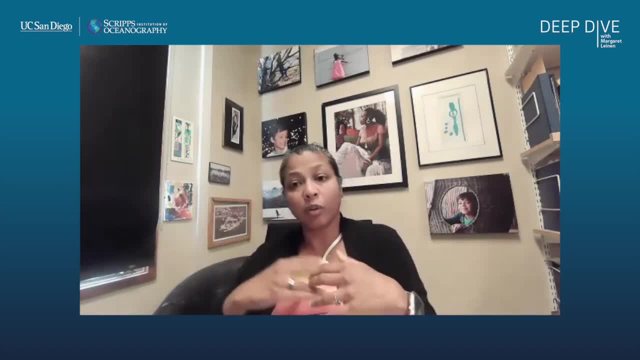 of these organisms, like marine mammals, where they've you know. you know, you've gone through many steps in the trophic food web. we see them in in relatively higher concentrations, and so that suggests to us that they're being biomagnified for some reason, or maybe they're being transformed. 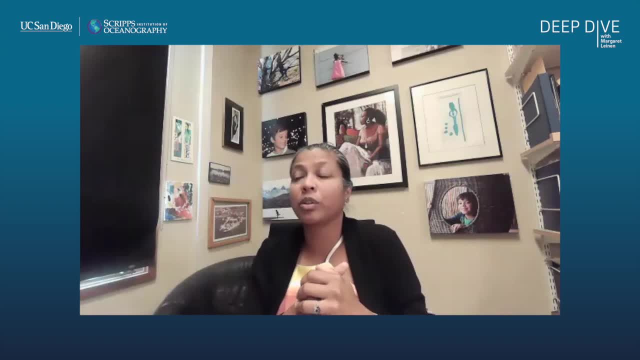 something is being transformed and turning it into what's in the technical mixture. but if we didn't look for that or if we didn't find that, we wouldn't know that it's having a kind of a it's. it's not a parallel pathway, right it's. it's sort of doing something a little bit different than 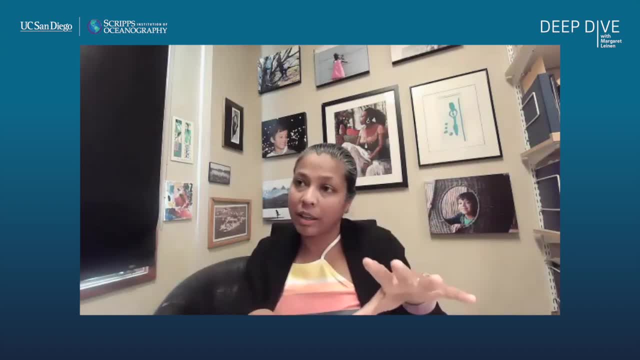 some of the other DDT compounds and if we really want to understand- you know how, what- what impact these chemicals can have in the environment. we really want to understand you know how, what impact these chemicals can have in the environment. we really want to understand you know how, what impact. 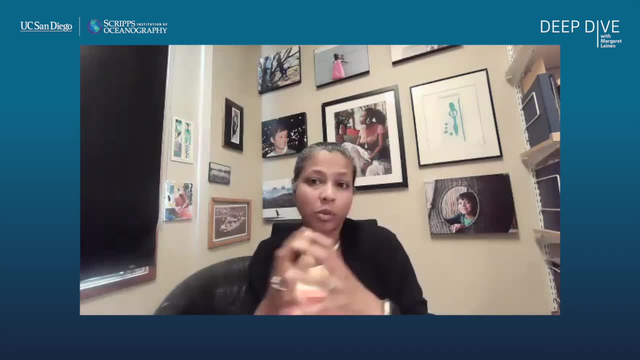 you really need to be able to look at them on a molecule by molecule basis, because their structures are different and so they behave differently through the system. so that's another reason it's really important to be able to look at the whole instead of just kind of you know it's. 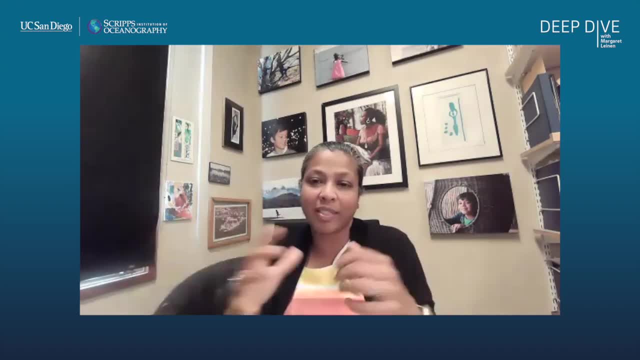 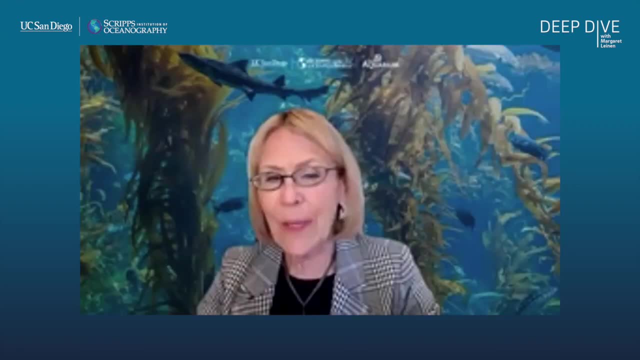 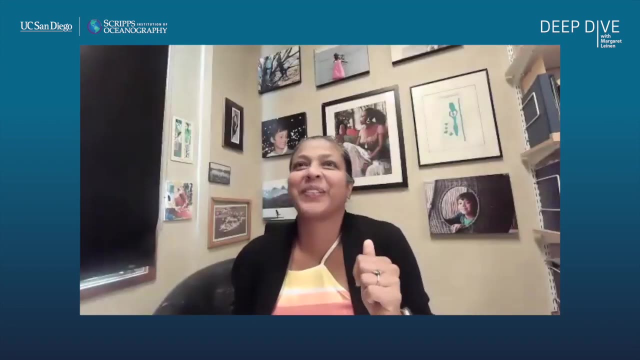 like I know. the analogy everybody uses is the, the blind man and the elephants. right, if you only touch the tail, what would you know? so, yeah, so you mentioned that you look in marine mammal blubber. why do you look in the blubber? yeah, because it smells really good. um, it was actually when we were doing this project. it was. 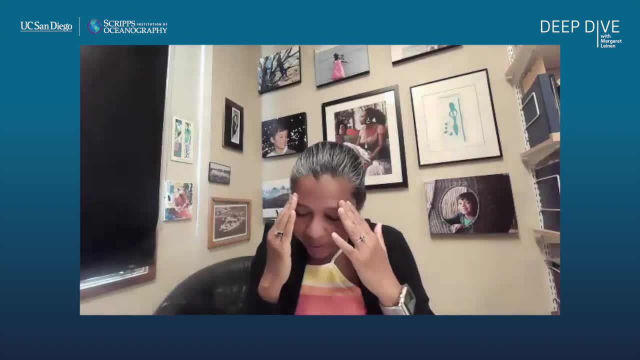 very sad. this fin whale washed up um in um. it actually on mission beach, and so, because we were connected to this project, we were allowed to come and take a sample and that's the first time I've actually ever been in a place, in a, at a site like that, where you've got, you know, they basically. 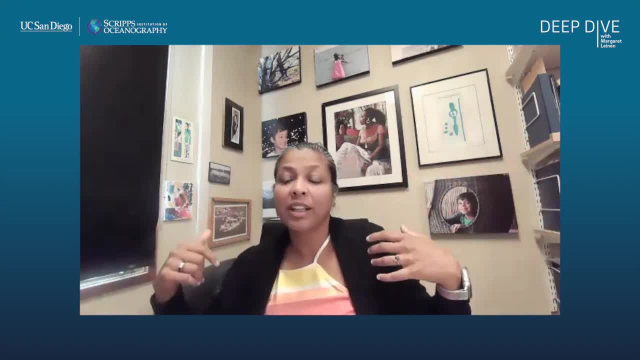 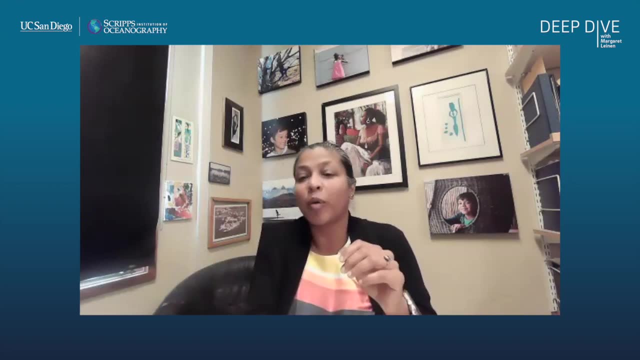 it was huge, right. so they had to bring bulldozers to pull the animal on shore and then they were cutting up the blubber and and that was- yeah, I was. I'm glad that I only got one gram blubber samples for the other analyses, because it wasn't that fun to we. 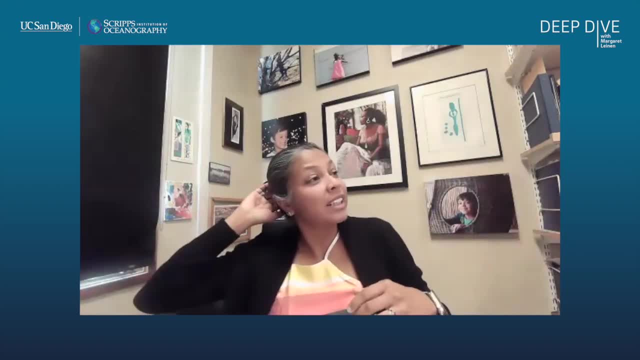 literally had like slabs. we had like a 50 kilogram slab of uh blubber from the fin whale, so the blubber is. you know, one reason we look at marine mammals is, of course, they are at the top of the food chain, so they're, they're apex predators and they, and we specifically, 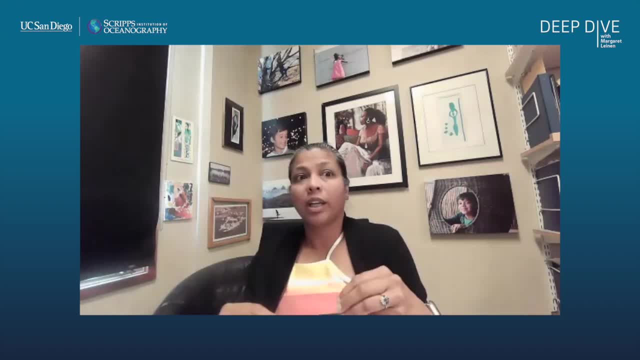 want, or animals that also eat other fish. so you know, if you're feeding pretty low on the food web, you're not going to accumulate these compounds. uh, to the to a great extent. so. so one reason we look at them is because they're apex predators. and then the, the blubber um, is a place where a lot 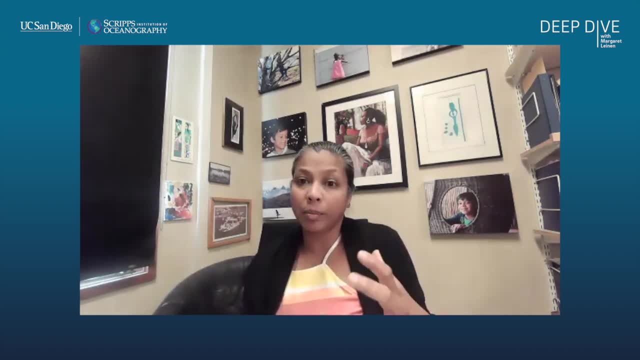 of these anthropogenic contaminants um accumulate because they're you know, this is a question people often ask about DDT related compounds. they're sticky, they don't want to be dissolved in water, so they're going to go. they're going to stick to particles and in an organism they're going to. 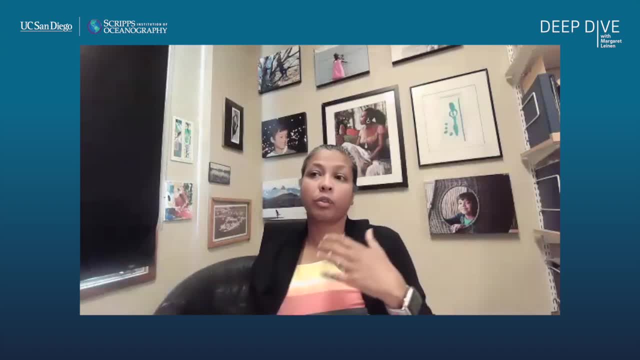 partition into the most fatty tissues that they can find, and so the blubber is the place where these things really accumulate, and if we want to get sort of a more comprehensive picture of the anthropogenic fingerprint in an environment, that's a great place to go, because there are a 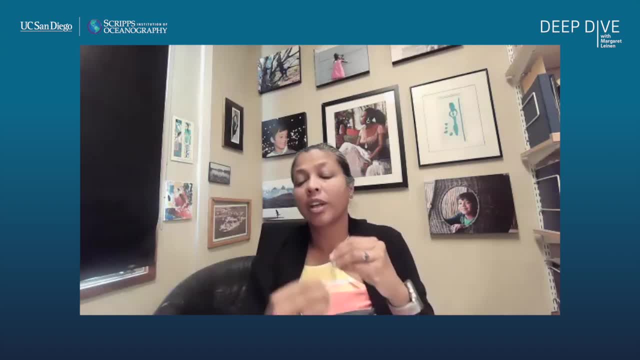 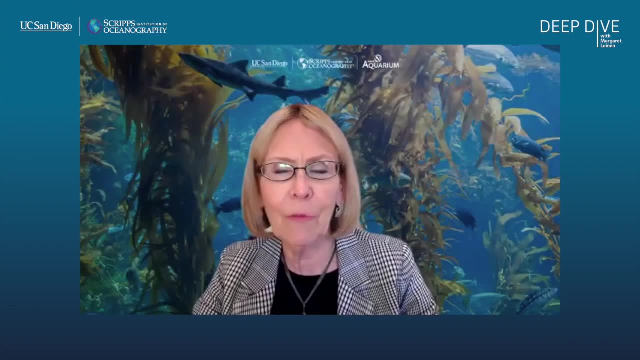 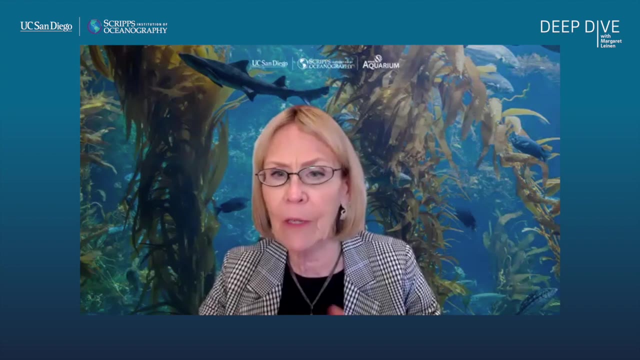 lot of these compounds are present in high enough concentrations that we can actually detect them. so you mentioned uh DDT and then briefly mentioned uh flame retardants. uh, are there other uh class? so I think people are familiar with the fact that both of those have been banned. uh, are there other? 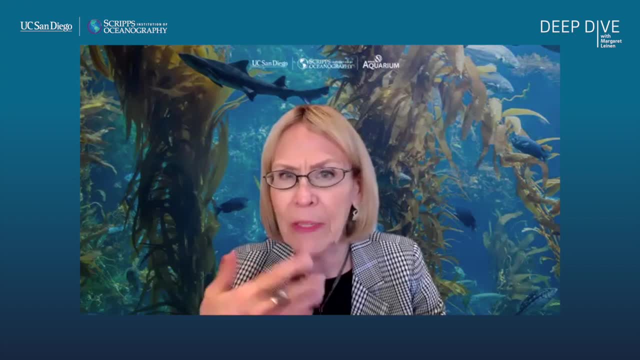 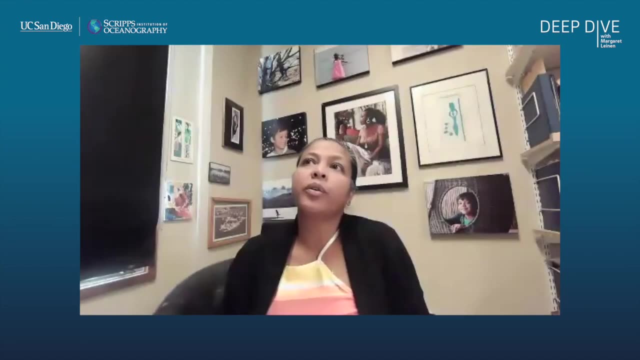 um, uh, organics, you know human generated organics that you see regularly, that are used, yeah, so, um, I think so. so there has been a a ban on the perfluorinated compounds of PFAs and we see a lot of interest in those because they are. 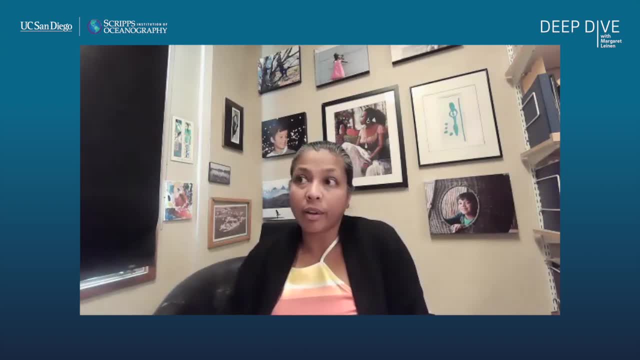 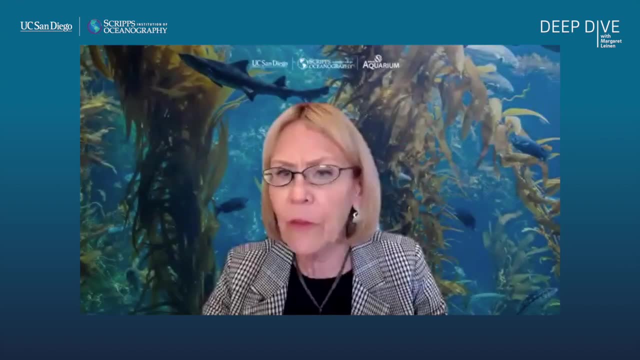 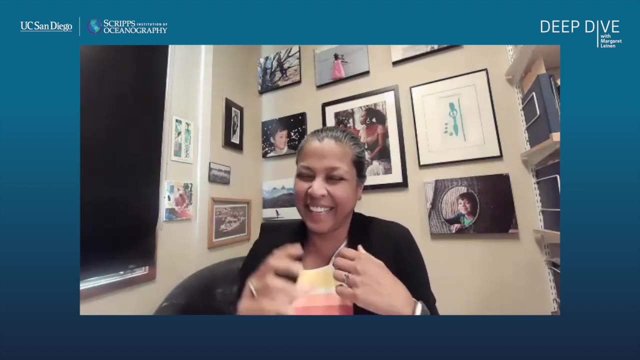 also incredibly persistent, and they are in the waste. they get discharged in the wastewater. so we see that in in the coastal environment. um, there's another. what do they come from? um, they are used. oh, that's it. oh, why can't I? sorry, I have a brain, I'm trying to think. 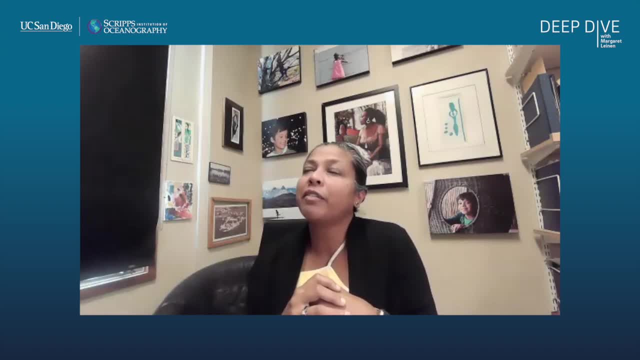 um, they're, they are, they're used in industrial manufacturing, but I, I think they're sort of they use, they use them as a coding for something, but I, I have to look it up, I can't remember. sorry, um, and I was just talking about this because we 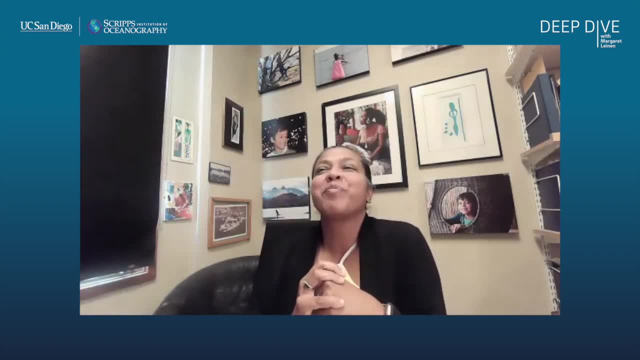 just have it in a paper, but just um, um and so. so there's- yeah, so there are PFAs, um, and they do. we see it a lot, but one of the concerns is in drinking water, but we see it in the wastewater, and then there are some other compounds that we've been seeing lately too. that, uh, different. 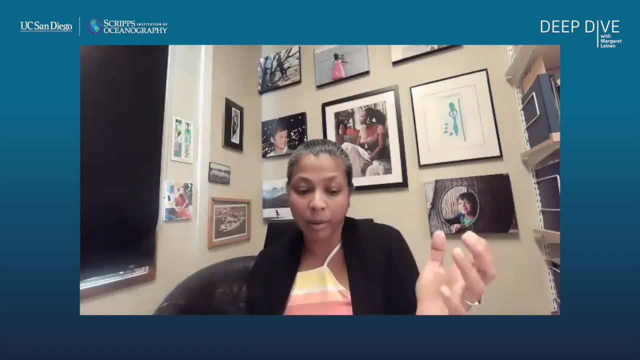 versions of these are their, their aromatic compounds through their benzene related compounds that are used in in in the manufacturing of the rubber in tires and that's a. it's a sort of an emerging um contaminant. it's been detected in a variety of different places and some, some of 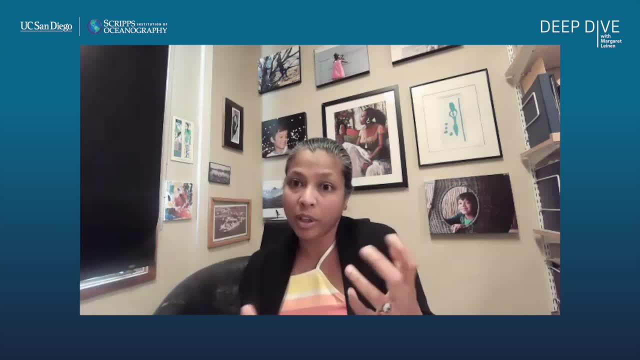 the chemicals that are found in these tires actually are transformed um through photo chemistry in the water to form dioxins, which are very potent. they're known to be that some of the potent dioxins are known to be some of the most potent um compounds um in terms of their toxicity. 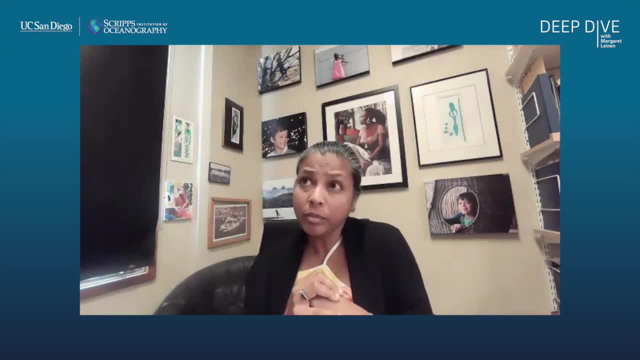 and those have been shown. they've been linked to um, um, uh, um, the. they've been linked to um growth, um inhibition in salmon, and so those are actually becoming emerging contaminants as well. um and so. so those are two of the ones that seem to have some currently um a lot of interest in them, because 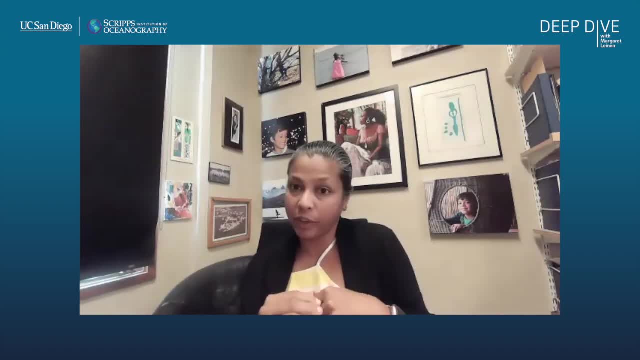 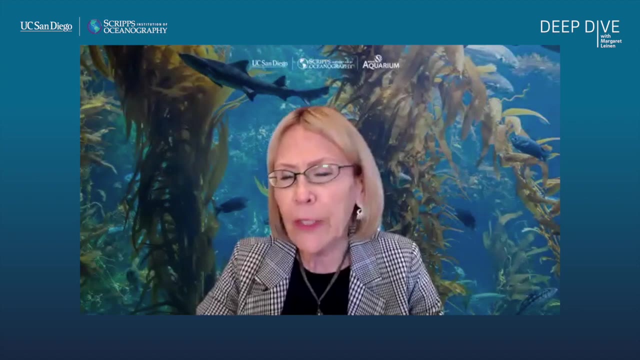 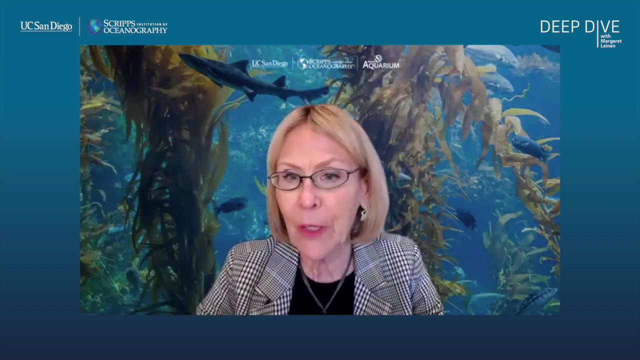 they're being detected at relatively regular frequency in a lot of these water monitoring um, um endeavors and we see, we see all of them in our- like the our time series off the pier, for example. so you've been talking about DDT a lot and, uh, just recently we found that there are many uh barrels of uh what we think uh. 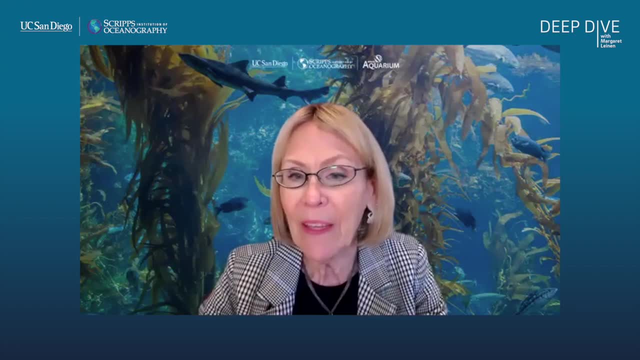 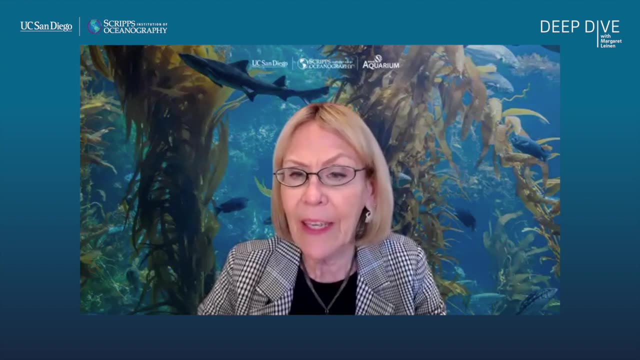 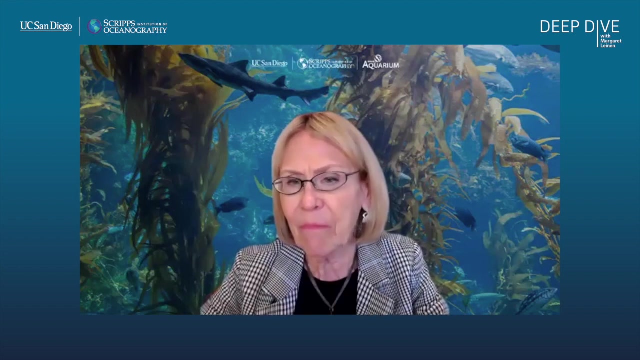 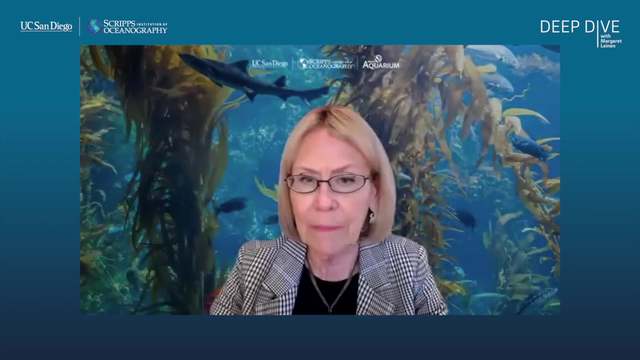 are barrels that we think are full of DDT um offshore of California and uh, some papers published about that and how uh is this also something that you're working on and how has that um affected your research? yeah, it's something that we're definitely thinking about and involved in. you know, when we first did the characterization of 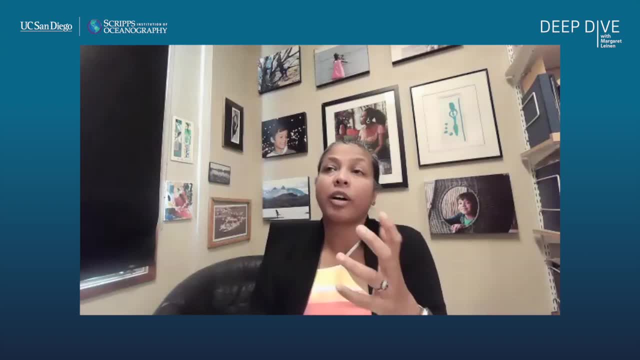 the DDT suite of compounds um in the dolphins, um we you know, we we know of the historical Superfund site of palace Verdes where Montrose, you know, basically discharged through the White Point's outfall DDT into the sediments and so we were familiar with that um dump site and you know the bottom line is the DDT is in our current food. 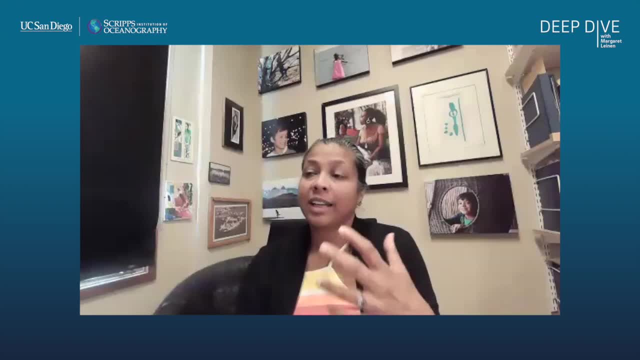 web right. so, regardless of of what the Superfund site has done, you know there's DDT in our food web and so we, originally, you know, know, we, we assumed that that was the main source and um, we also know, you know, people use the ddt. 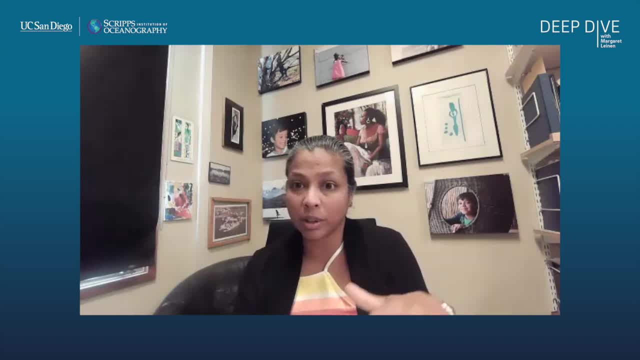 concentration in marine mammals that migrate all over the world, as a indicator of the fact that they feed off of southern california, because we're talking about orders magnitude higher than any other location, at least in the us, for ddt um. so this rediscovery of the potential for 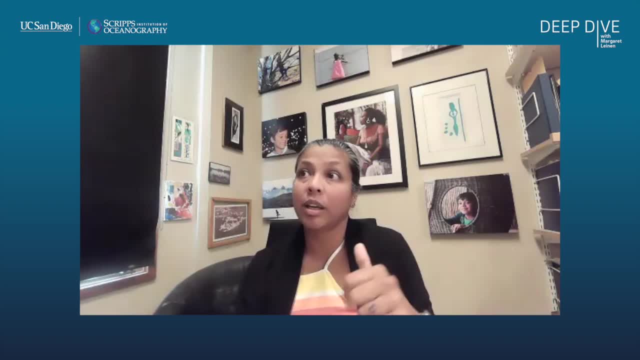 hot for at least comparable amounts of ddt being in the sediments off in these, in this deep dumping site, the dump site too, i think, in in san pedro basin. you know that makes us wonder. okay, well, you know. uh, you know, maybe there's, there's another input of ddt into the food web and what's. 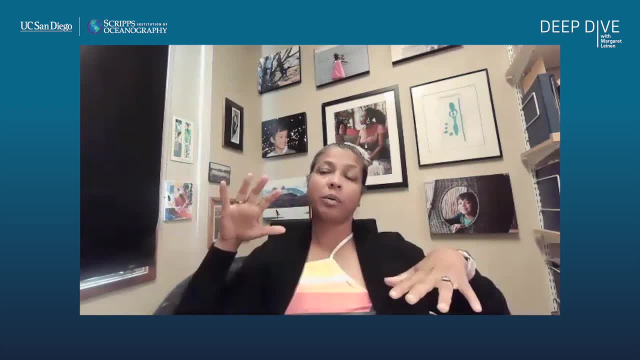 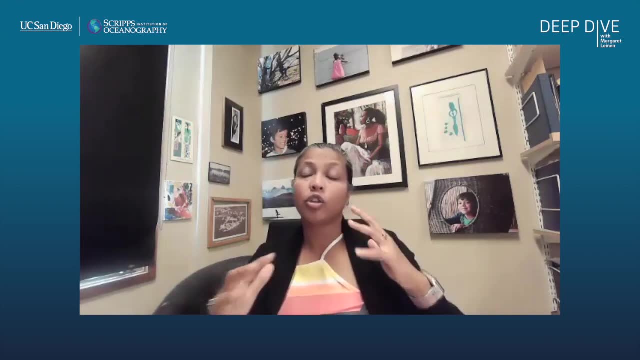 been interesting to us is that, you know, in our dolphin study, we looked at inshore feeding dolphins and offshore feeding dolphins and we didn't see- you don't see- a significant trend, uh, in terms of um concentration or body burden between those populations, whereas you do see it for some of the other things, like pcbs, for example, and so it's not. 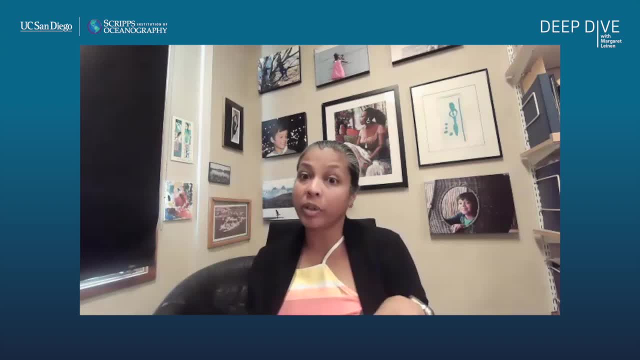 to say for sure that that's a smoking gun, but that was something that we had recognized previously and several of unha's papers subsequently has has also noted that, and so that, might you know. that raises the possibility that in fact the ddt in the offshore site um is entering the food web, and i think that's, you know, that's, that's always something. 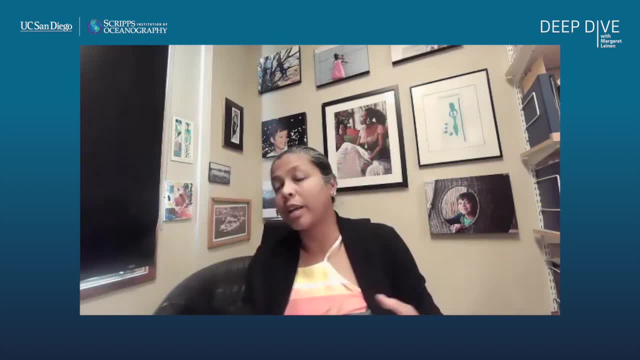 we've wondered, because the ddt, does you know, it will end up in the sediments. so how it gets into the food web is really an important question to answer. but the other thing that we wonder is whether there's, you know, the ddt barrels, or at least what's purportedly dumped. there is the waste. 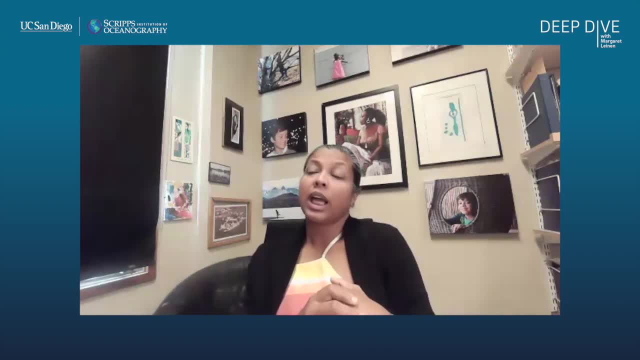 from the industrial manufacturing process and so you know there could be a pretty unique fingerprint associated with how that material is moving through the food web. and that's something we're really interested in, because we have these innovative tools that can kind of- um, you know really where the complexity is accessible. we can kind of we can capitalize on that to really try to. 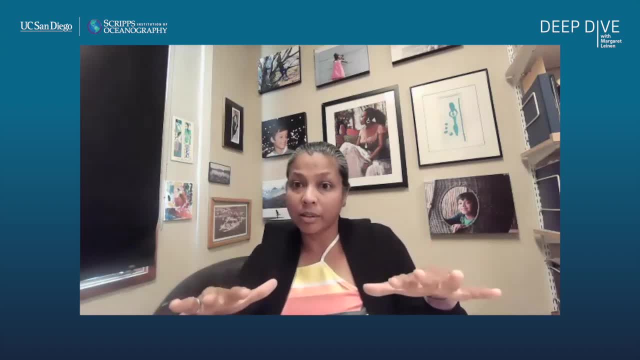 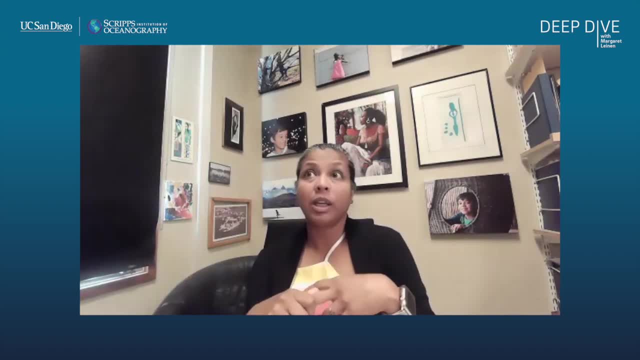 different locations. so that's what we hope to do- is to be able to characterize the fingerprint of what's in the sediments, or hopefully, even if we could get access to what's in the barrels and see if that fingerprint tells us something different um than what we would expect to see. 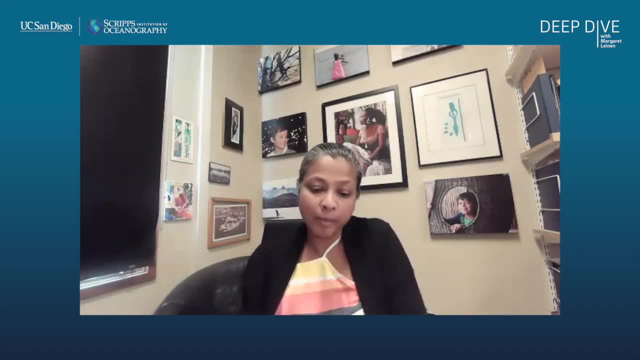 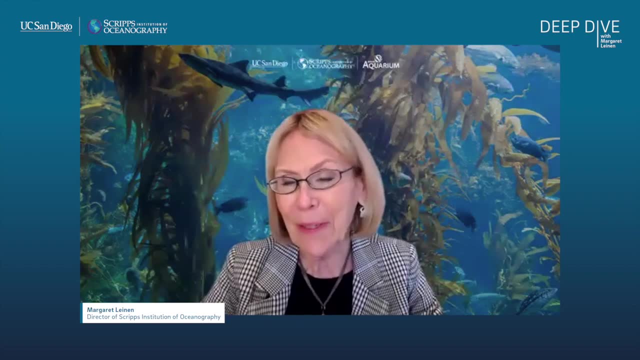 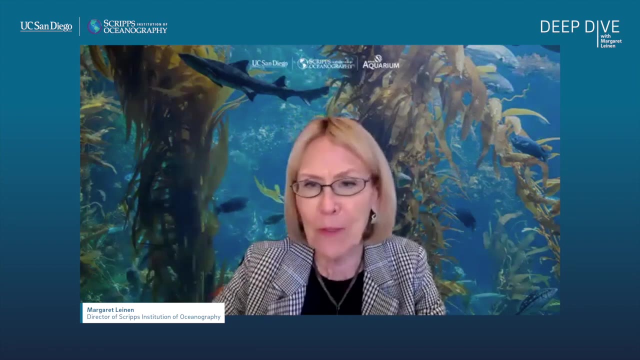 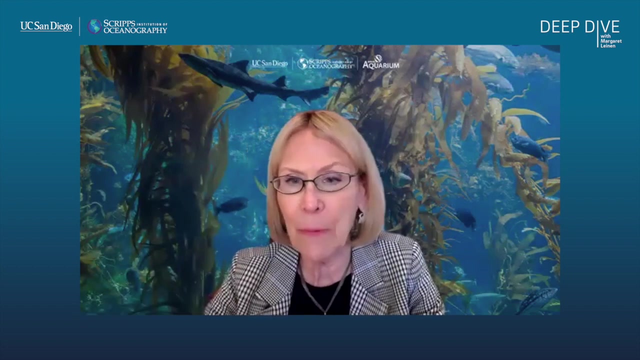 from the palace where they site. yeah, um, as you think about chemical oceanography and your uh, your area of chemical oceanography, and look into the future- you know sort of 10 years, beyond 10 years, whatever- uh, what are the big opportunities that you see there? what do you think that people will be uh doing with with this uh in the future? 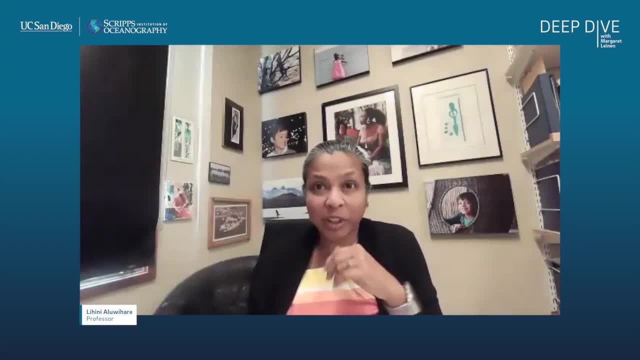 yeah, um, you know, that's a great question and and there are lots of different types of chemical oceanographers who probably prioritize very different things um from me. but you know, one of the reasons i got into this field was i was because of the importance of of organic matter. 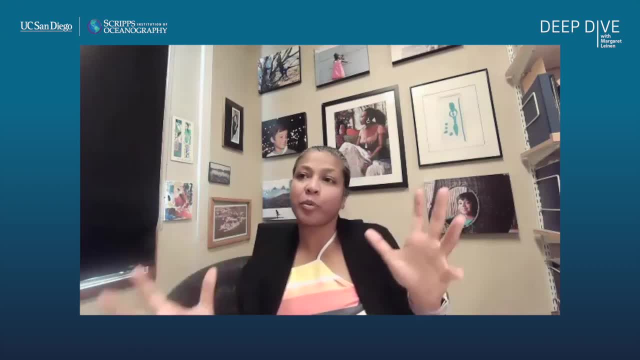 in the carbon cycle, right, whether it's uh- transport of carbon in sinking particles out of the photic zone, whether it's these- you know we talked about these long-lived versus short-lived compounds, and so i think, um, you know, we we talk a lot, we are, we talk a lot about the 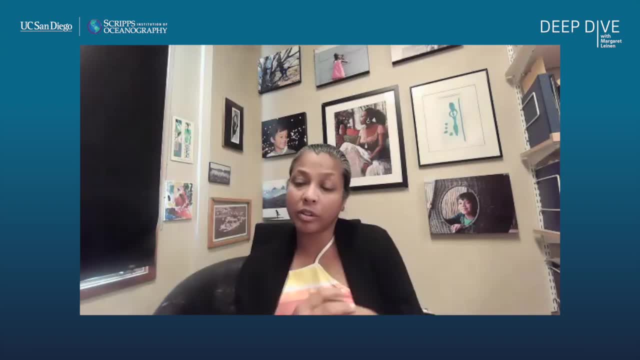 factors that influence how much its carbon is fixed by phytoplankton in the ocean. but i'm really interested in what impacts kind of the removal of it, what? what are the environmental and community composition level changes that impact the respiration rate of carbon, whether it's in the 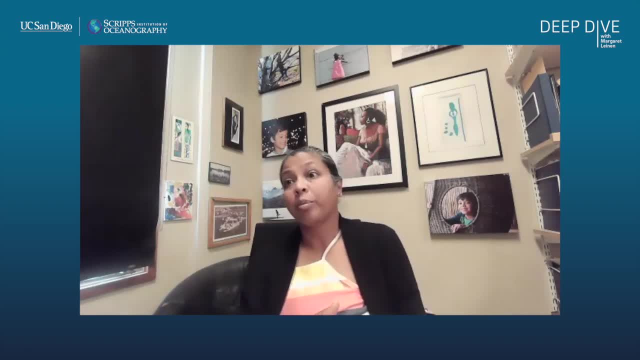 surface ocean, but also in in these low oxygen environments, and there's a lot of renewed interest in these low oxygen environments, especially in the water column, because you know there's a lot of interest in these low oxygen environments, especially in the water column, because you know, because there's, you know, with climate change there's the possibility and there's some evidence. 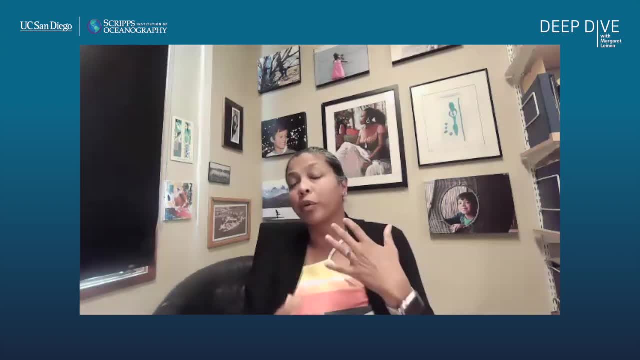 that suggests that they would expand, and so how microorganisms function in those environments to respire carbon versus, you know, allow it to like, allow it basically by not working on it to preserve in the environment is something, um, that i'm interested in studying and and um and very um. 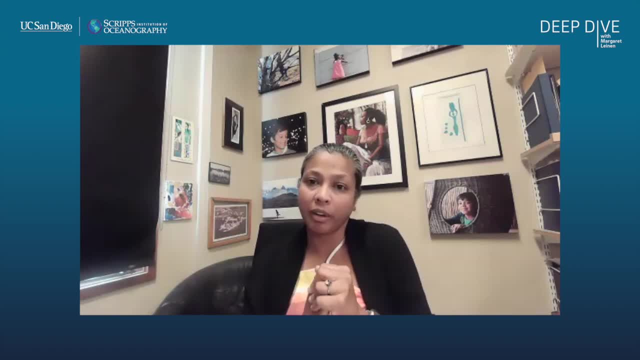 and and we have some work going on in those areas. i think another big question is that fate of terrestrial carbon as it comes into the ocean, and that's also not a new problem, but now that we see how land use change and warming in the high latitudes has mobilized a lot of this carbon. 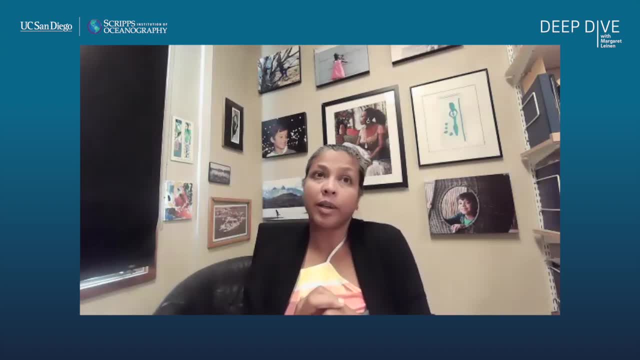 bringing it into coastal environments. this is a very important question. we really need to quantify how much of that carbon is being turned into co2 or methane and released into the atmosphere. essentially, you know, provide acting as a positive feedback to the warming versus how much of it is either getting. 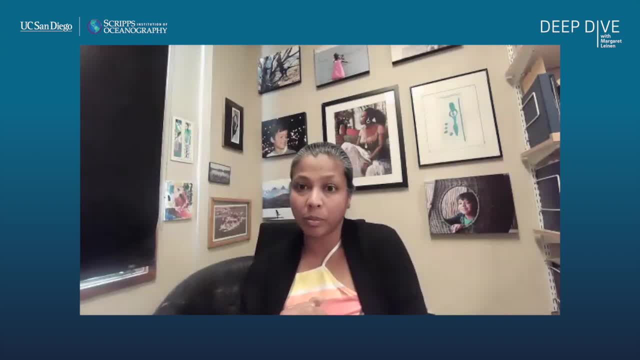 exported into the deep ocean or being transformed in some way, and so i think that that again, is a problem that lends itself well to some of the tools that i'm developing, because again we have to be able to look at molecular level changes, and then we also want to couple. 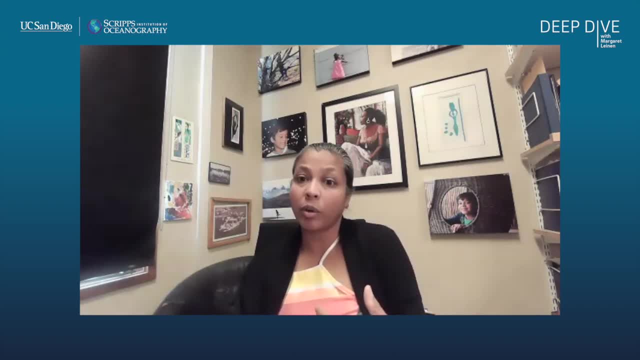 with isotopes, because some of these carbon stores are actually quite old, and so we should be able to to differentiate those from using radiocarbon techniques. so so i think- um, those are two, you know- looking at the the way that respiration rates in the ocean are being impacted by climate change. 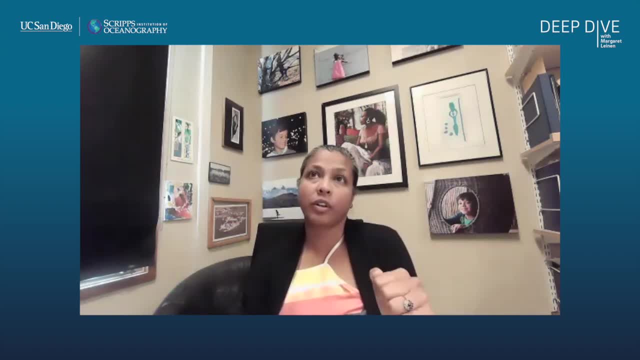 and changes in oxygen concentration and then the fate of terrestrial carbon, and i think this is an important thing to also consider, because we know that things like peat, but also wetland carbon, is a very potentially really important future source of carbon, of carbon sequestration or locations. 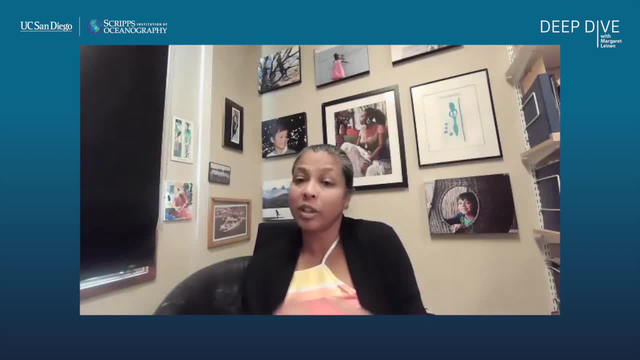 where we can sequester carbon because they actually have a really high capacity, these waterlogged sediments, both in tropical peat and these coastal sediments. So trying to understand what determines the respiration rate of that carbon and how to tweak that to increase storage. 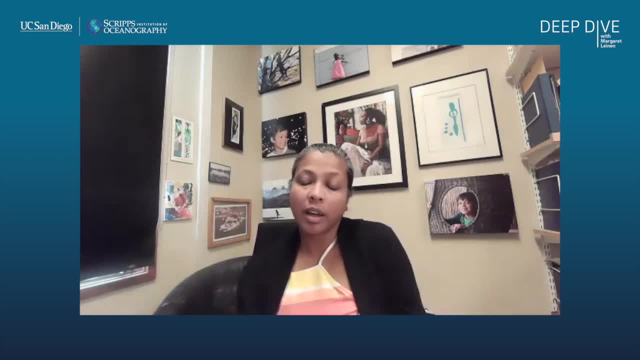 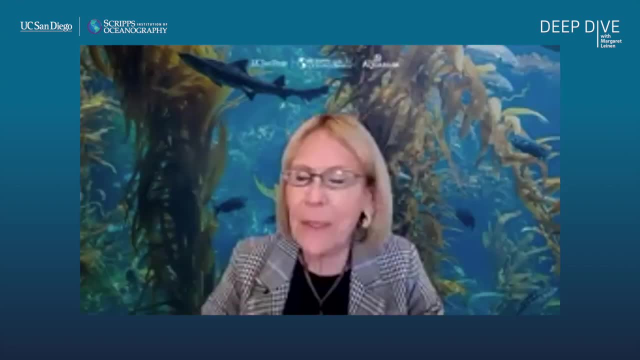 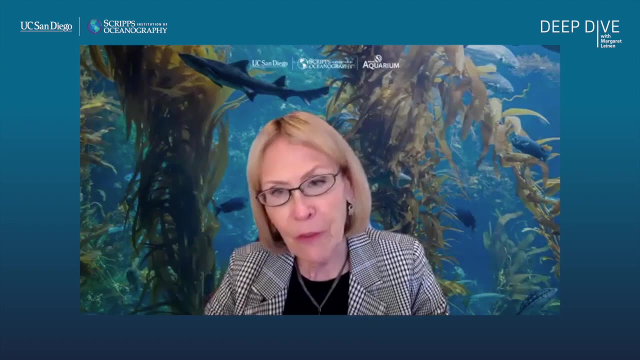 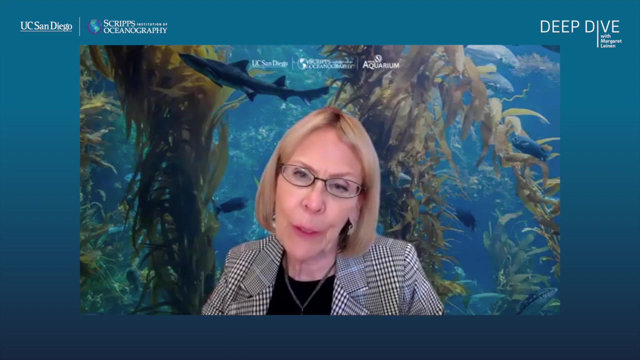 I think has ramifications that go beyond just the discussion of terrestrial carbon transport. So at the beginning of our conversation I mentioned that you have done really so much work to help us diversify Scripps. Why is diversity important for science, Right? I mean- 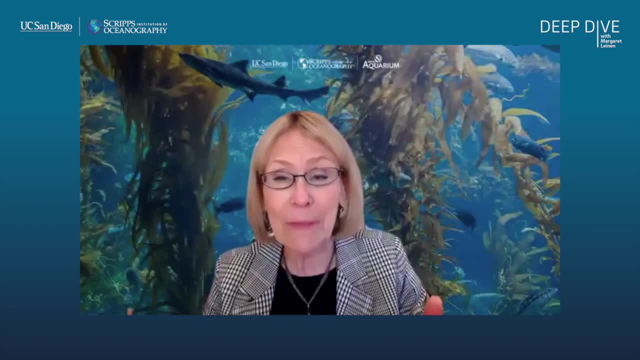 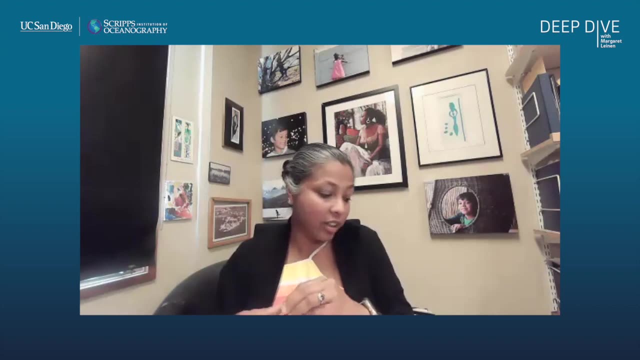 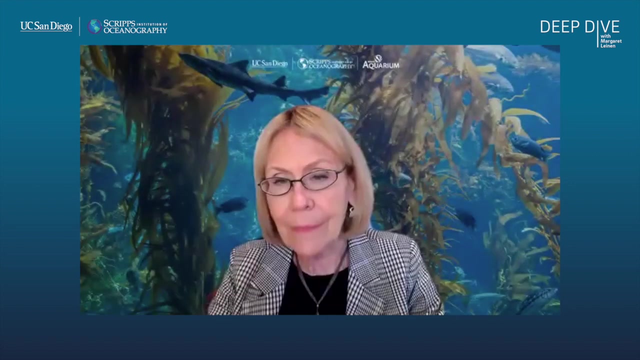 It's important socially right. Is it important for science? Yeah, I think you know the easy answer and I think it's the correct. it is a correct answer, which is that having a more diverse group of people involved in the enterprise. 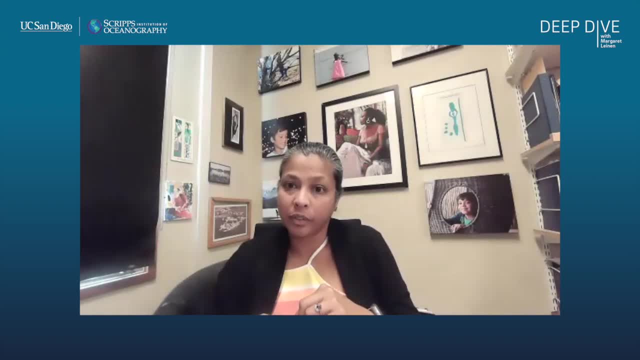 means that the type of products will be different. right, The kind of science that we do. But I think it goes beyond that right If we don't have people with the lived experiences, the cultural sensitivities and the cultural competency that underrepresented individuals bring to science. 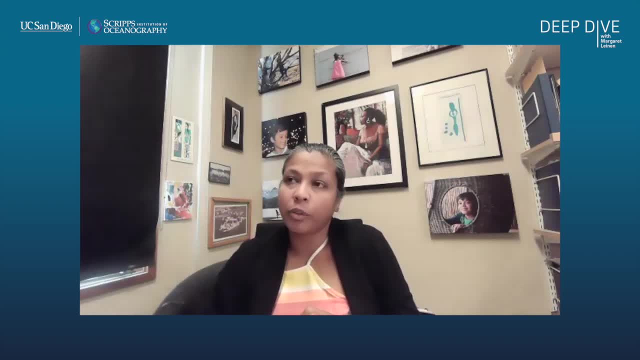 there are gonna be problems that we aren't even thinking about as being important, right As we. you know, the climate problem is a great example, right. Any climate solution that doesn't center the dignity of poor people or the dignity of black and brown people. 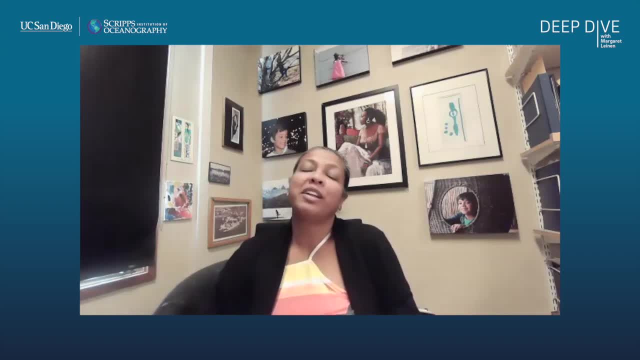 is not a climate solution. And if we don't, you know, many of us can read books and become educated, but the lived experiences and the cultural competency is crucial, not just to identify, identify what kinds of scientific questions and how to do science differently. right, I think. 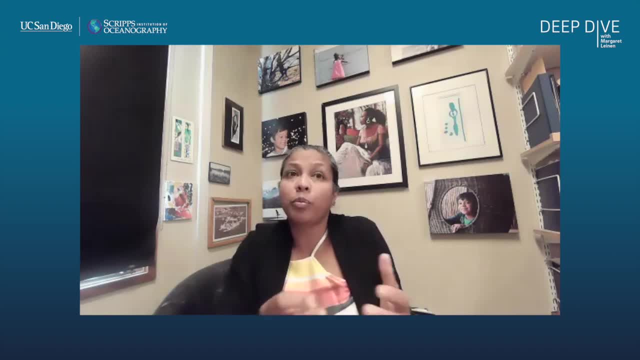 that's a key thing that we have to keep in mind. Science has been done in a particular way because of the people that were involved in it, and as we change, who gets to get a seat at the table, science is going to evolve, and it will evolve in ways that are probably very relevant for what's. 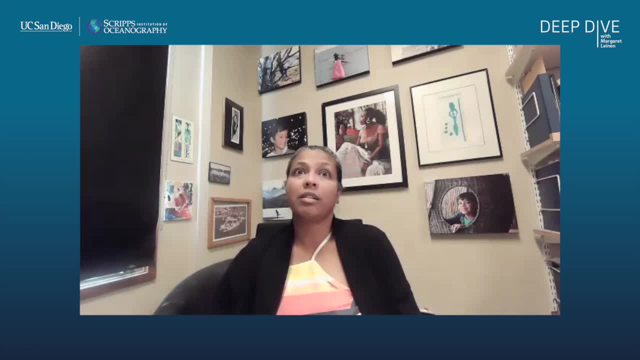 happening in the world today, but it also means that we can train the next generation of scientists differently, and so I think it's not just about, you know, having diverse minds. work on a problem might come up with diverse solutions, but it's a transformation of what we will be doing as 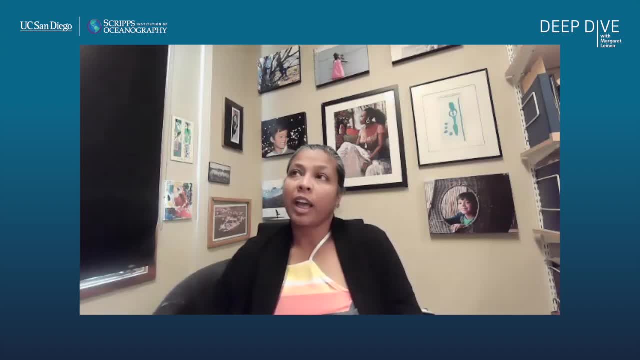 scientists going forward and you know it's really. I think it's difficult work. you know it's. there's no age index, you know, for that kind of effort and it's uncomfortable, It makes people uncomfortable. 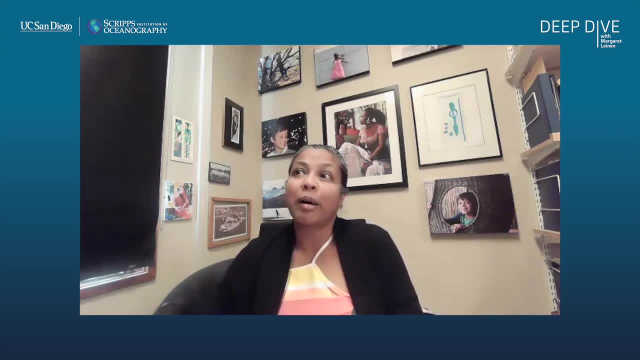 but it's really important that we think about what it's going to take for us to evolve into the 21st century as earth scientists and ocean scientists. For any non-academics out there, what's the age index? Well, just you know, it's how many people read your papers. essentially, That's basically what it is. 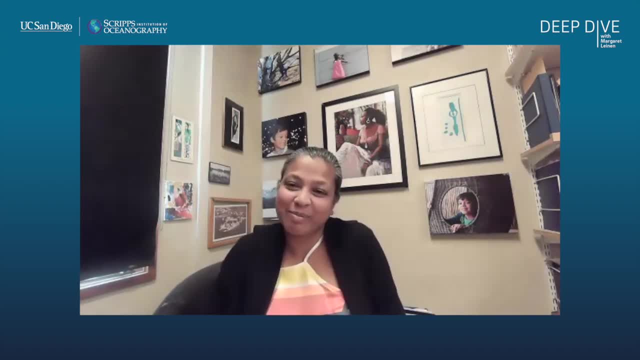 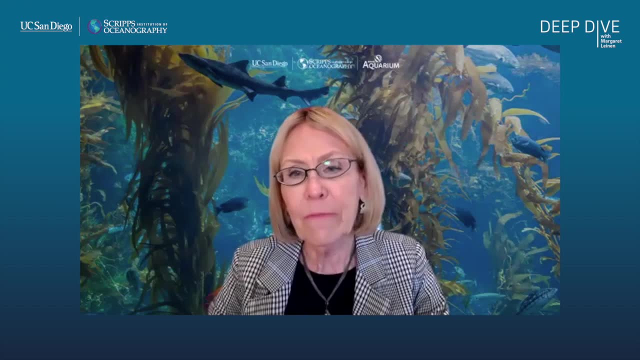 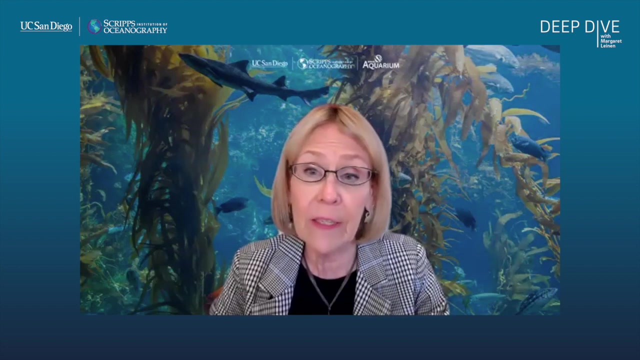 So, yeah, Yeah, it seems to me that it also. you know, having diversity in science and in the voices that we listen to is also important for how well people trust the science. If it's not relevant to you or if science has overlooked major issues that you see, I think it's important to. 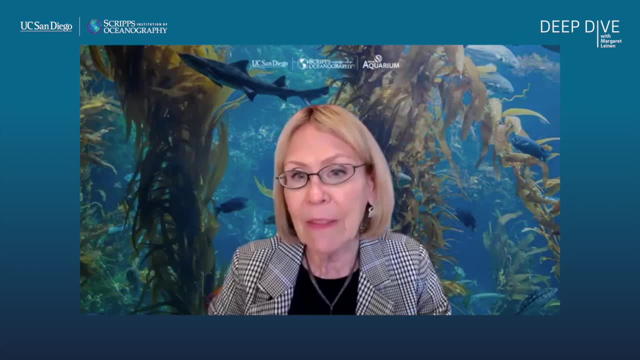 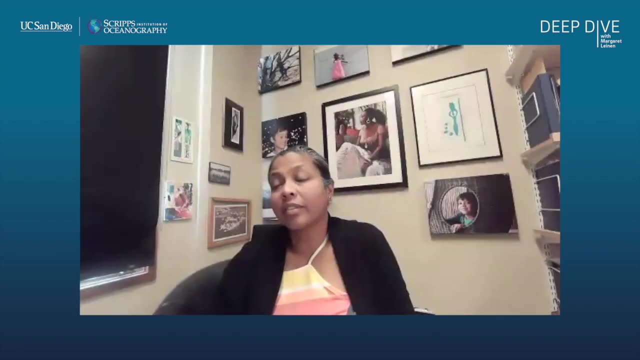 see as being relevant, then you know. you may say: well, they don't even know this, Why should I trust them? No, that's exactly right, and I think that's you know. you articulated that well and 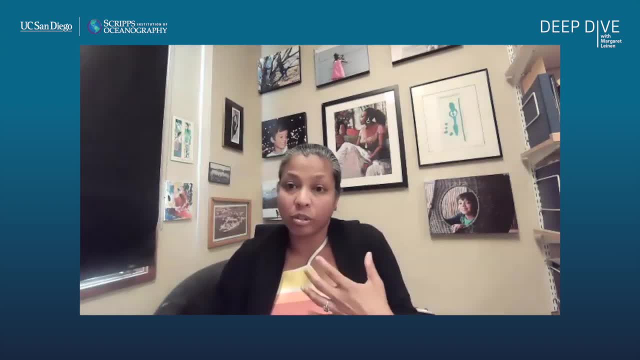 that's what you know. that's why I think the climate solution issue is such you know. this is why it's so important to involve all these different voices, because that will require everyone to come along. right. That will, and the fact, you know, rolling out the COVID vaccines. 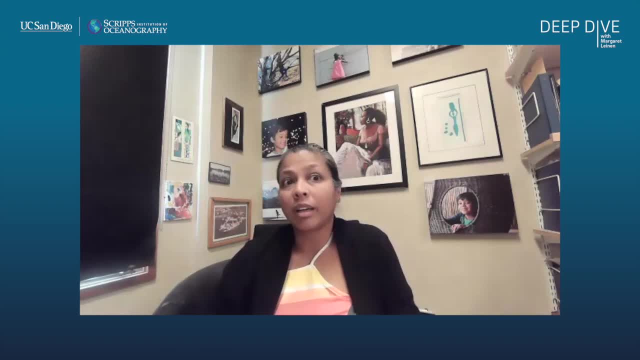 is a great example of where it's really important. I mean, and in health sciences we've really seen that play out right in a lot of different ways. where it hasn't been very inclusive, That has influenced what kinds of you know medical conditions we focus on. but it's also influenced 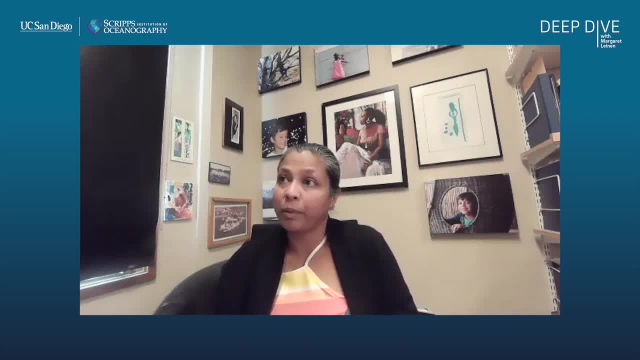 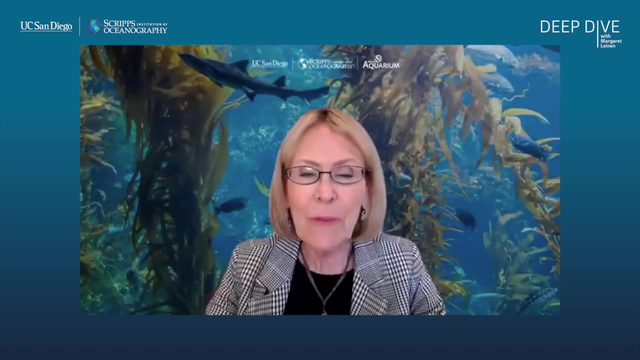 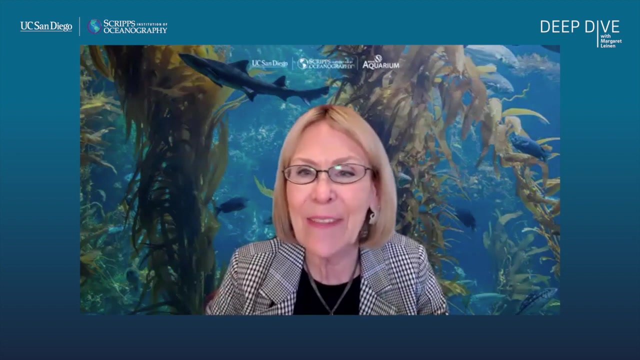 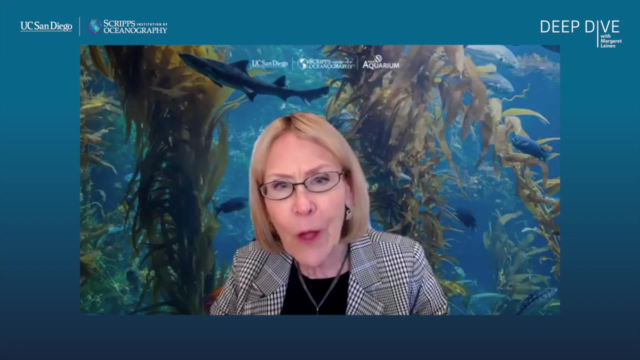 how efficiently we can convince people to trust the system, as you put it, with these vaccines. So yeah, it's a really good example. So I'm enjoying looking at the photographs behind you and I see children and I see some beautiful art and but I don't see any pictures of dogs. 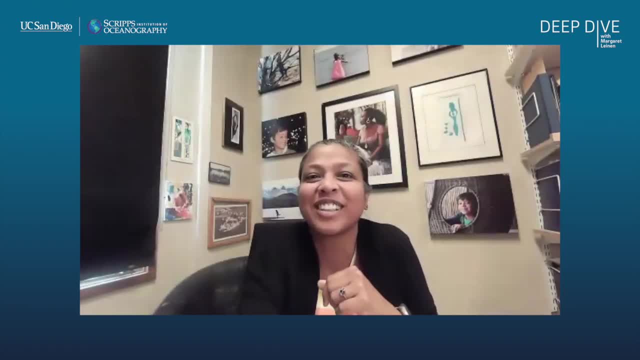 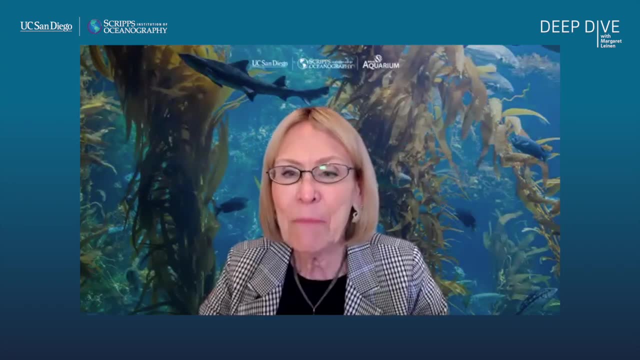 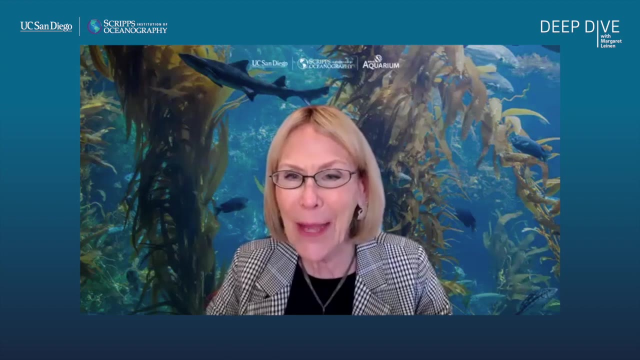 and I'm surprised. Well, yeah, Everyone at Scripps knows that you foster. There's one, Oh, there's one. So everyone at Scripps knows that you are. you are the foster mother supreme for dogs. How did you get into that? 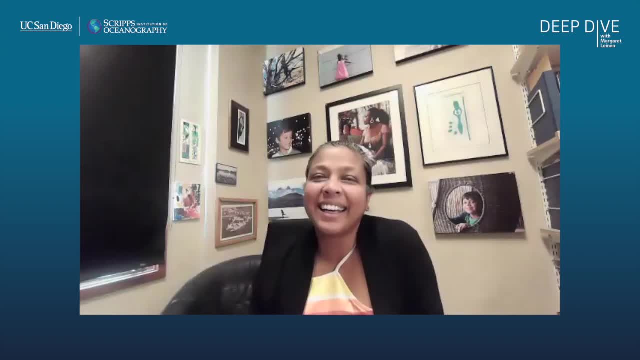 Yeah, so I had. there was a former graduate student at Scripps, Ashley Corrigan, who runs the rescue that I work for. It's called the Rescued Dog and you're lucky I'm not at home today. 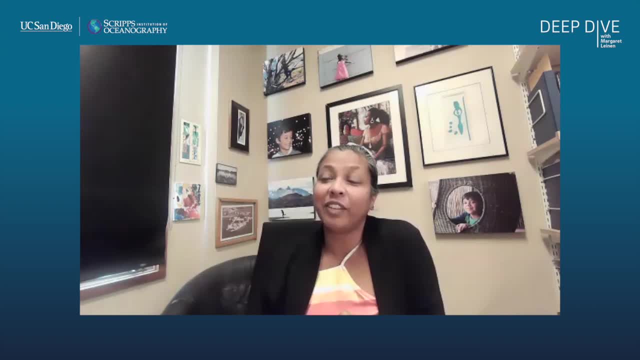 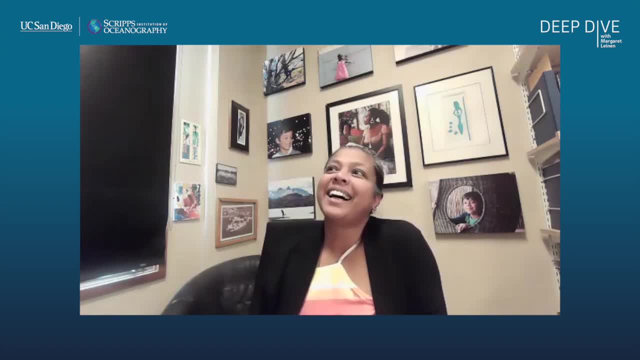 my gosh, Oh my gosh. I'm fostering them right now And I lost my long-time dog, who is actually in that picture, and I had said to my husband that you know I was going to go to the pound and find a dog and you. 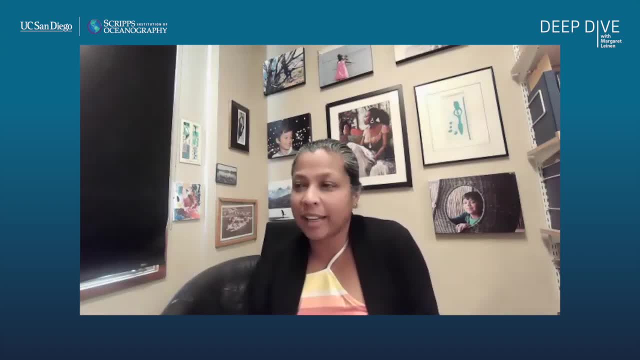 know, I don't. you know, I'm going to bring it home, and even if it attacks my only child, Roahsshaan, I was still going to keep it, because that's what we do, And so he thought he was. you know we were having this conversation. 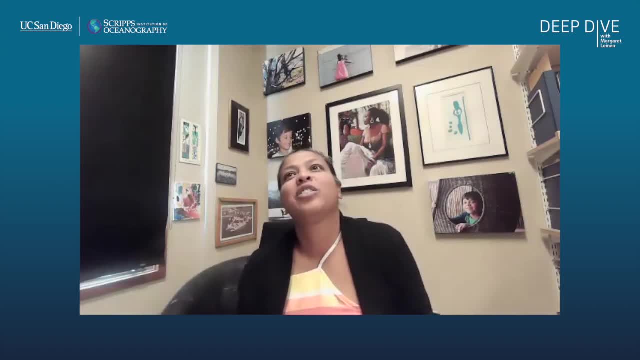 and so one of my former graduate students, Jananne, suggested that look into fostering and she put me in touch with Ashley, and so that's how I first got into fostering dogs about seven years ago and, yeah, and I've been, and I you know, one of the things I found really 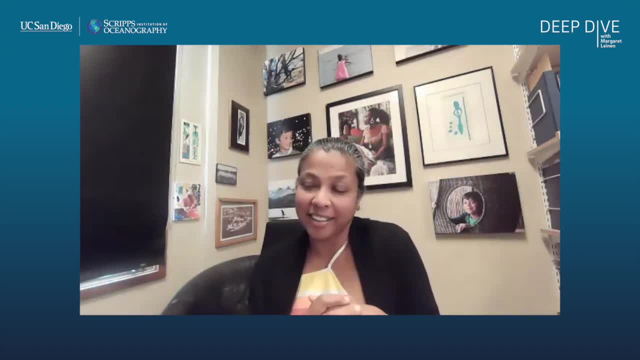 funny was that the first dog I fostered, I decided to adopt him, and so they call you this foster failure, and I was immediately offended by that and I was like, no, I don't fail, that's not going to happen, and so so it was kind of like it was for my pride that I continued to foster and I'm 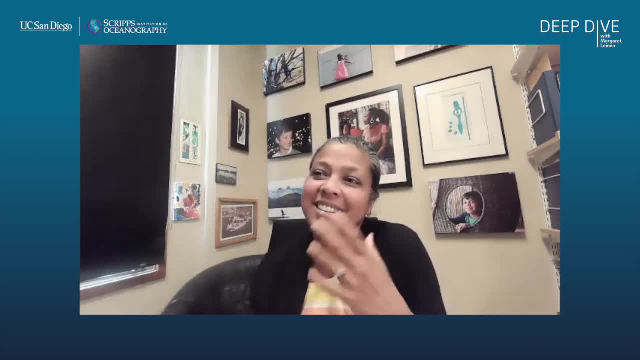 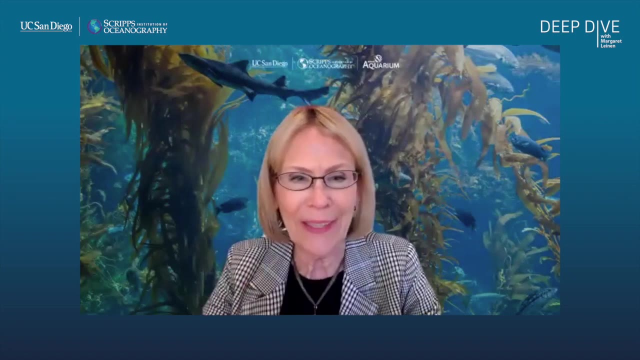 glad I did, because I I really enjoyed it. and then it just gives me. you know, it really changes my frame of mind when I go home and sit in a pile of puppies, even if they're covered in poop. well, that's organic too. yeah, exactly, that's part of the grand cycle, right? all those microbes. 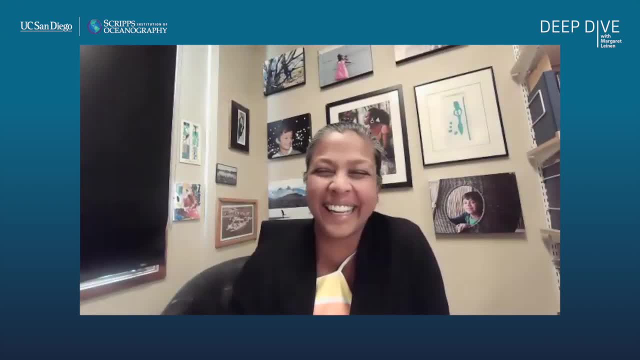 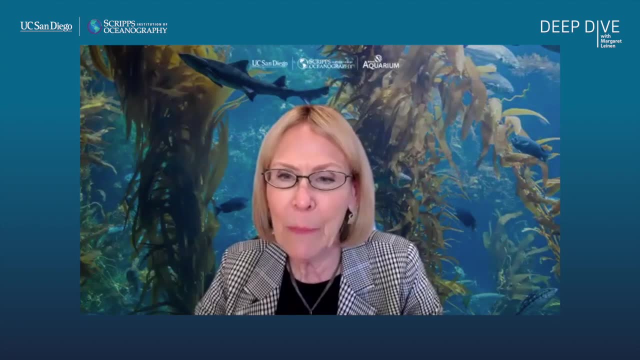 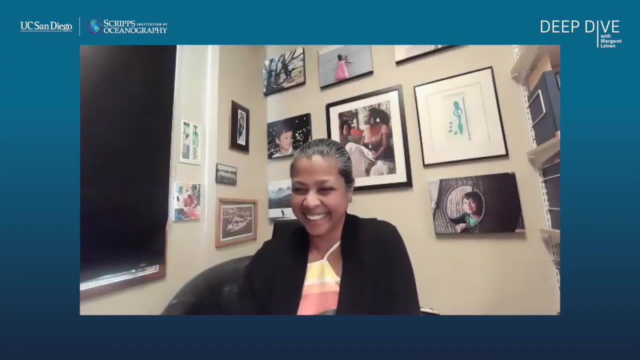 I'm glad you understood, understand- not many people do. yeah, well, as, as you and I have said before, the microbes rule the world. they just let us live in it because we're great hosts for them. yes, yes, indeed. oh, look at me. thank you so much. it's. 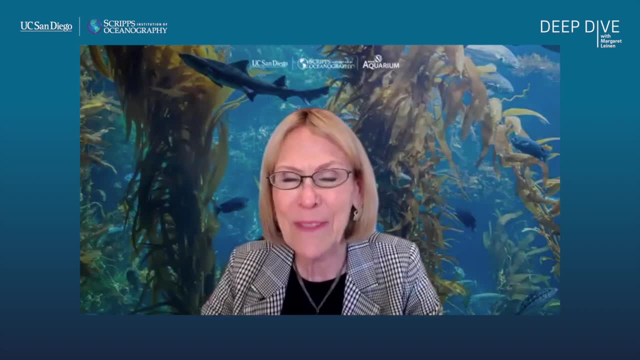 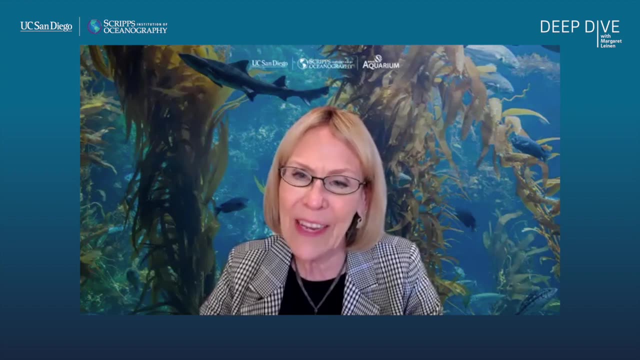 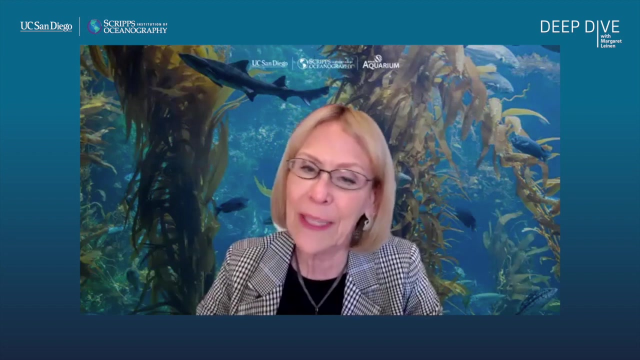 always a pleasure to talk to you and thank you for taking the time to do this little film so other people can enjoy a conversation with you and you can understand the um, the really interesting things that you can do with uh chemistry and with organic chemistry in the ocean and that it's really important for us you're looking at at. 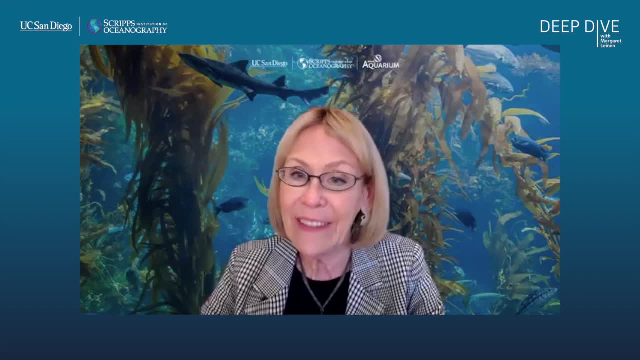 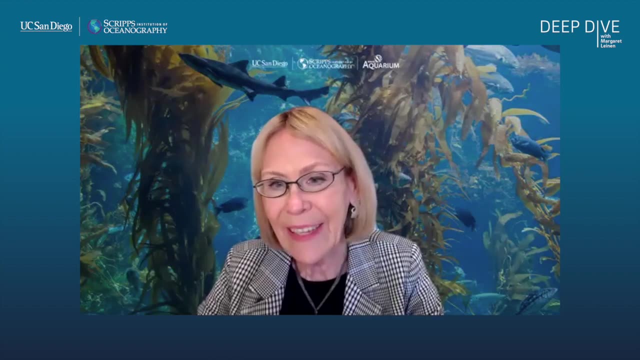 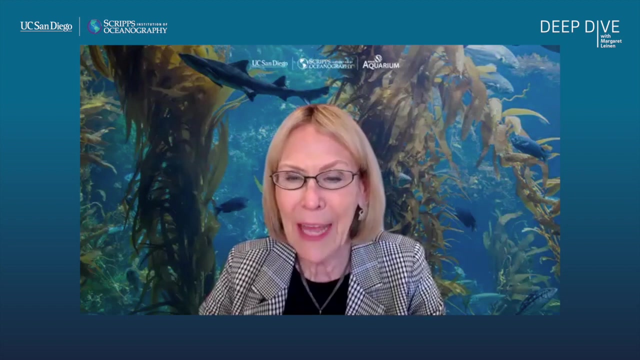 these things that are very toxic and, uh, you know, can move into the environment and, as you said, can be in our food chain, and, uh, we certainly don't want to be thinking about eating DDT. it's bad enough to uh have it around us. and also, thanks for all of your work on enhancing